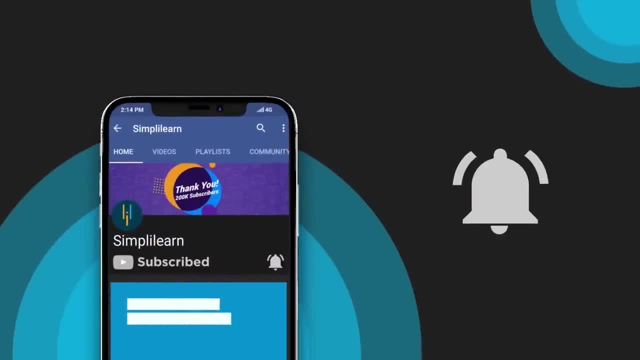 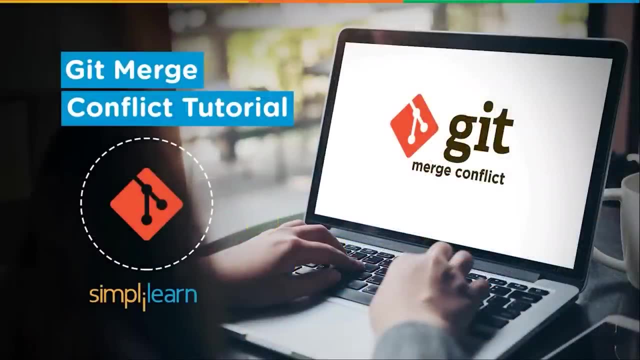 Welcome everyone to this lesson by Simplino here in which we are going to talk about the Git Merge conflict over this one. Now, we all have worked on Git and we know that Git is a very good version control system which we have all together. But how to resolve a problem which is known as? 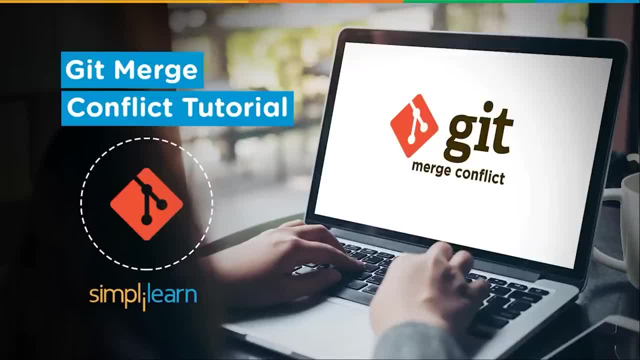 Git Merge, Because during the developers check-in or do any kind of merge activity, this is a common problem which they face on daily basis. Now, this is something which we are going to talk about in this, so that we can give an kind of an insight to all those developers and to other particular 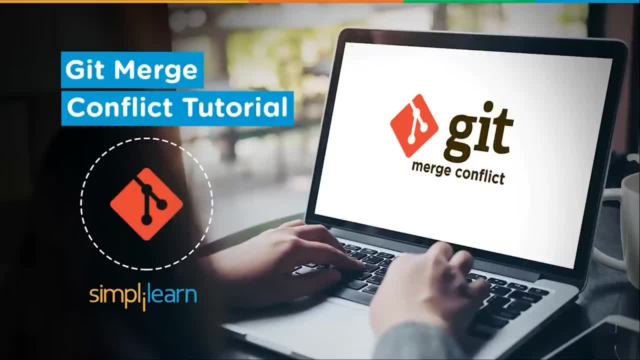 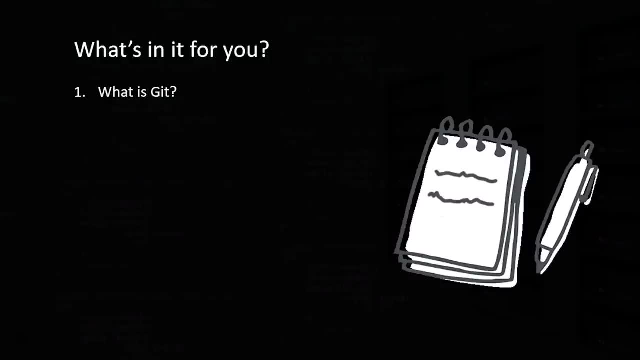 different people who are using the Git version control system here. Now, what exactly we are going to talk about here? We are going to talk about what exactly is Git version control system and what exactly is Git version control system. So let's get started. 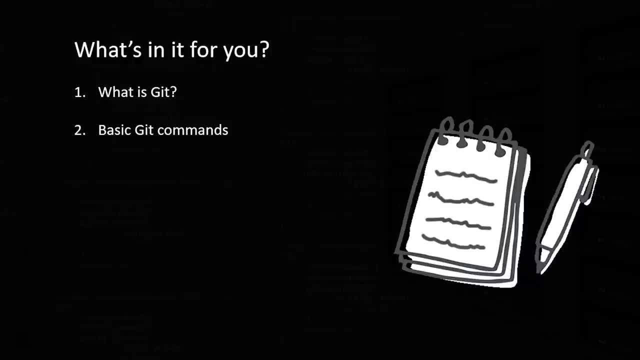 We are also going to talk about what exactly is the basic Git commands used in Git, And then we are going to talk about that. what exactly is a merge conflict all about? And then the different type of merge conflicts which we encounter while doing any kind of merging or any kind of modifications. 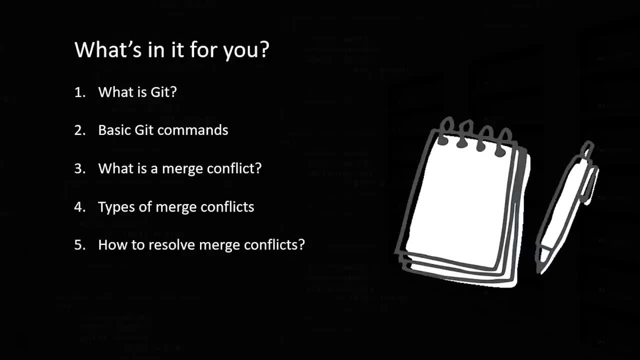 And then how to resolve these merge conflicts faced by a particular individual or a particular developer. And then the last one is how to resolve these merge conflicts faced by a particular developer. And then the last one is that the various Git commands, which is involved in resolving 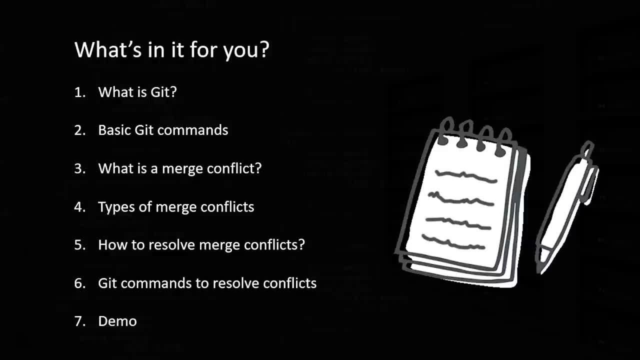 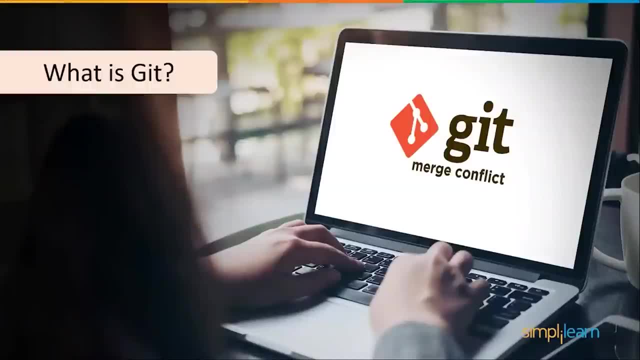 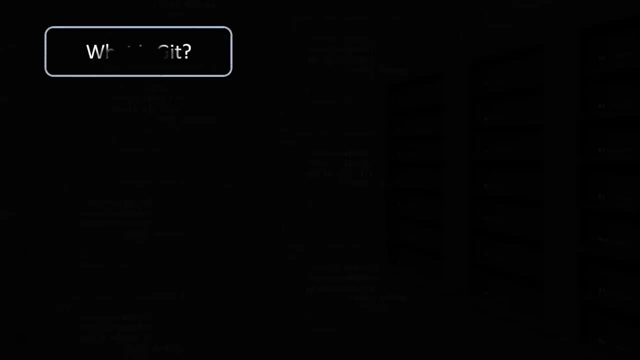 these conflicts, And then we will be going on with a small demo to better understand that, how these conflicts can be resolved all together, Right? So let's first of all talk about that. what exactly is a Git version control system? Now, Git is a kind of a version control system. 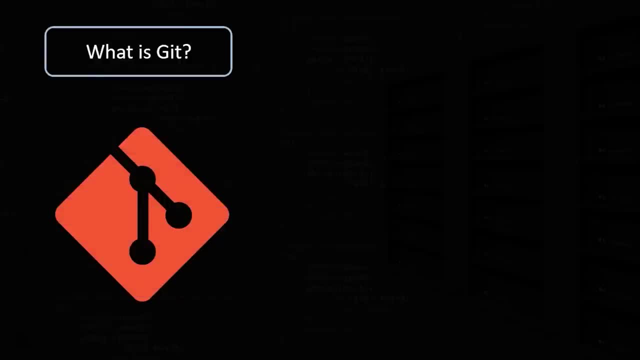 which we basically used for storing our kind of source code there, which can be used for storing a source code of Java, NET, Android, Nodejs. different kind of programming languages can be stored all together in this version control system, So in an organization. 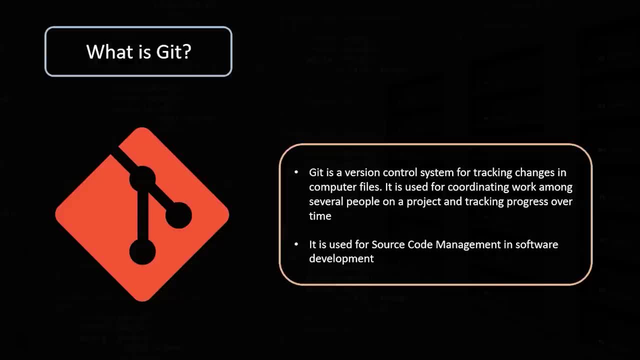 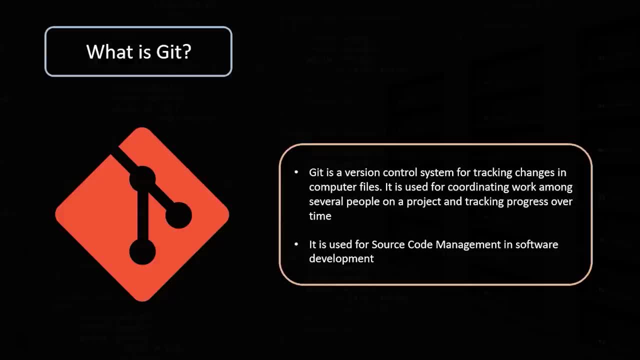 which is used by different developers, And in fact, it is not only limited to developers. a lot of other people also exactly use this specific tool. Now, the main task of using this tool is to perform a better coordination of the work here among the different people, among the 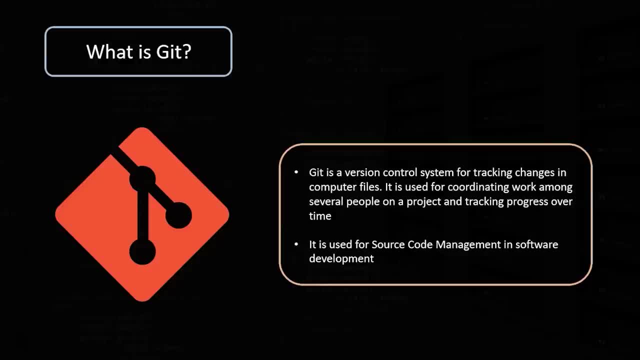 different developers and also to have a proper track of the particular progress of the specific project. So using the repository you can see that over the period of time you can do the tracking that how the different commits are happening here, how the different source code modifications are being done. So the complete status and the 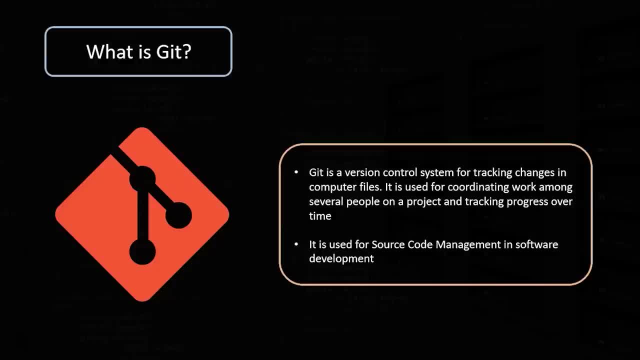 complete stats, you will be able to get from this a kind of a version control system here. Now it's mainly used for source code management here in a particular software development process or a particular team here. So it's a very important and in fact a 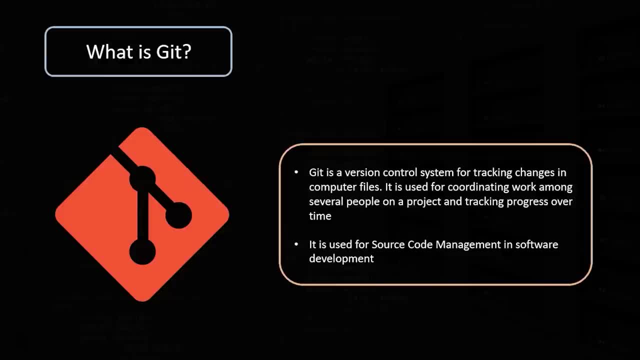 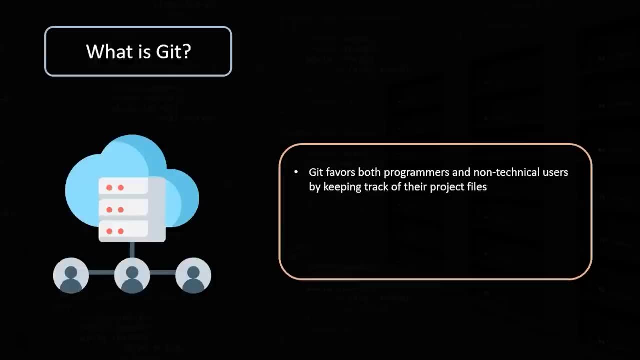 key tool for any kind of development project, So the development cannot survive without having a Git version control system. Now, Git favors both programmers and non technical users. Now, if you are a programmer, definitely you will be using it for storing the source code and having 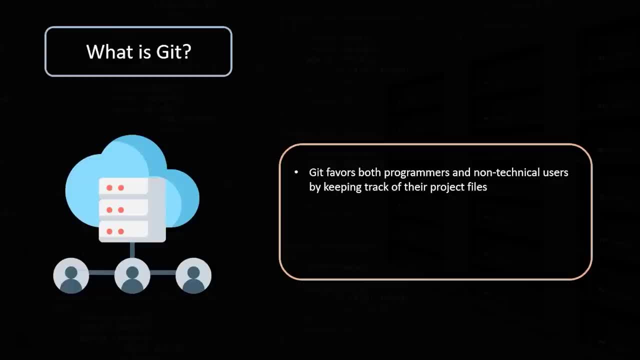 those particular files, having some dotnet source code, Java or some particular source code present there. But in fact, if you're not a particular developer, if you're not a programmer, you are working as a non technical job. So in that case also you can store it for keeping. 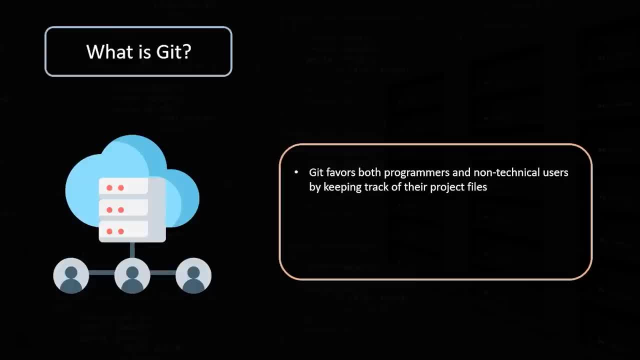 your project files. Best example: a particular DevOps engineer can also use these repositories to store their version control systems to have the scripts- Python scripts, shell scripts, configuration management tool scripts- any kind of automation scripts they can store. They want to have it. they can keep use of these particular version control system here. So it's not a dedicated. 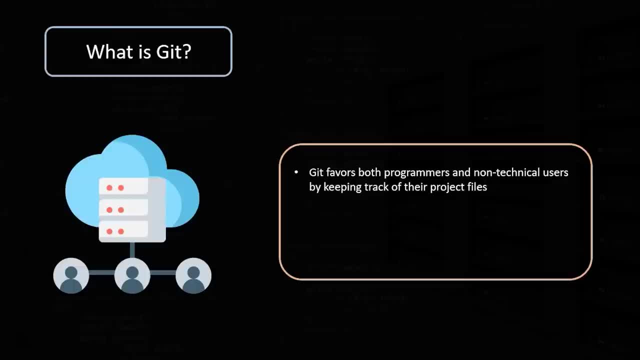 tool for a particular developers. Anyone who wants to utilize the features of version control system can make use of this specific tool. In fact, it allows a multiple users also to work together, So different people and different programmers can collaborate with each other with the help of this. 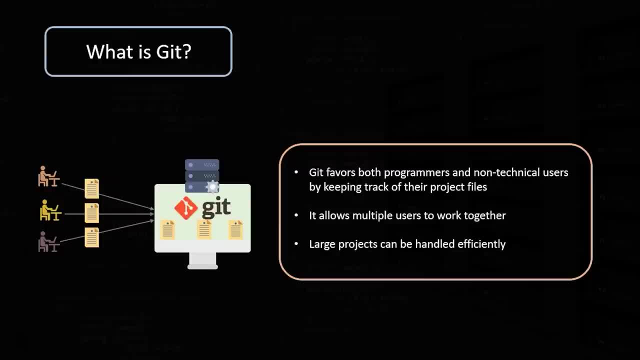 particular specific tool here, And it can also handle large projects. If you feel that you are working on a particular big project which is having multiple repositories, multiple projects are there, So in that situation, get version control system will survive and will provide you a better performance in different different aspects. 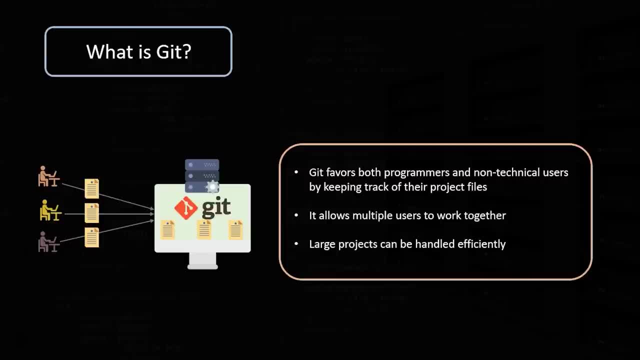 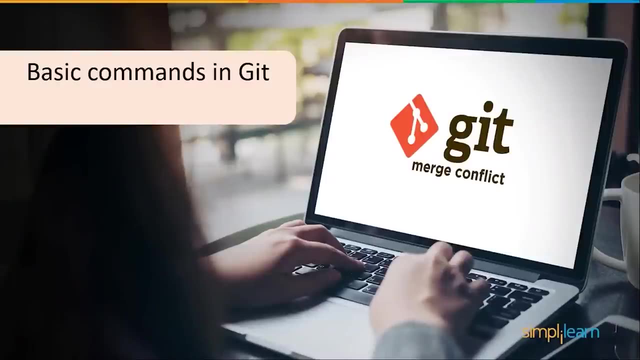 So it's a very good tool for you to handle big, big projects where you are involved with multiple changes, multiple programmers, multiple collaborators and different kinds of source codes. Now, what are the different basic commands which we use in git to manage a git repository? Now, 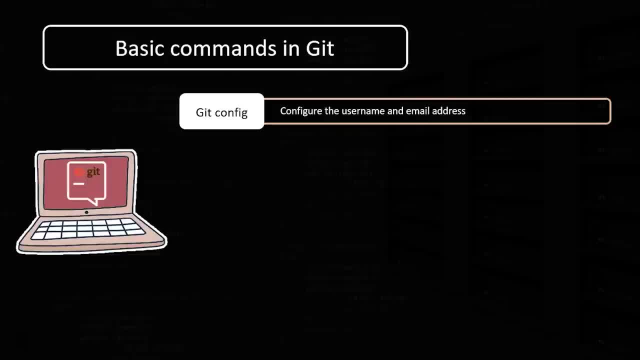 first of all, the very basic command of a git over here is git config. Whenever we work with any kind of git repository locally, when we do a git clone and we manage or we do the modification to the git repository locally there. So in that situation, 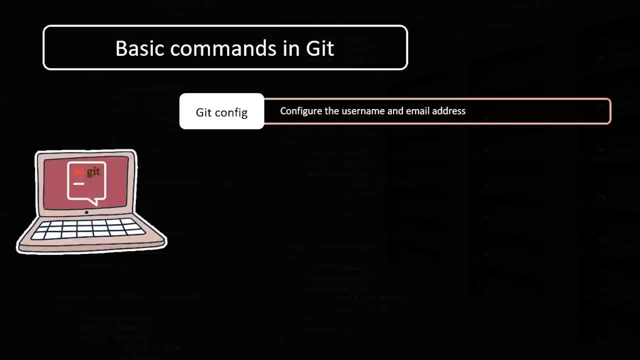 we often have to provide some details like the username, email ID, so that whenever we provide, whenever we do some kind of commits, the author details should be submitted according to that. So in that situation we have the particular command called git config, which will 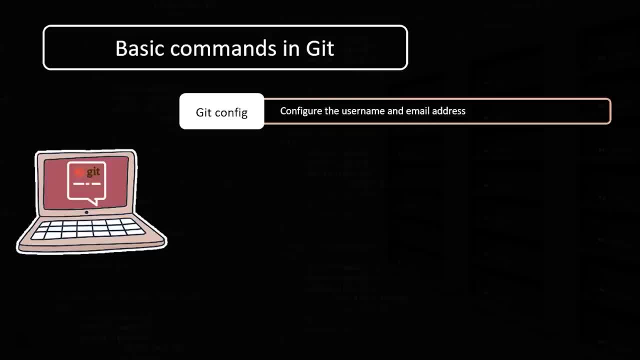 definitely help us to do some configurations so that we will be able to have some configurations configured and we will be able to have some author details or some additional parameters. so all those things we can configure using this git config command here now, if you want to initialize a local repository. 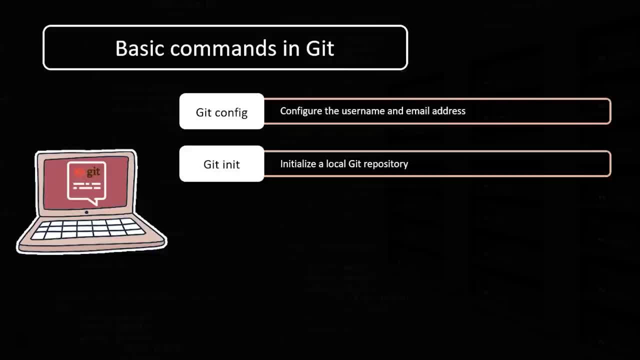 now you're not working on a remote repository and you want to initialize a local repository. in that case you can use the git init command in a specific folder so that you can convert that a simple folder in a full-fledged git version control repository. so init command is used to initialize a local. 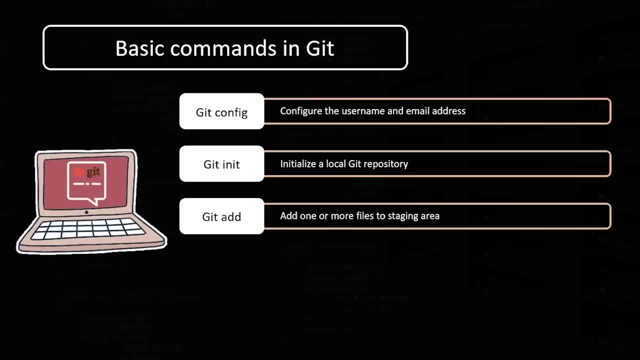 empty, bare git repository. next command is git add. now git add command is used whenever we do any kind of modifications into my local repository so that file will be present into the working area, into the working copy over there. now, the moment you run the git add command on couple of files or on 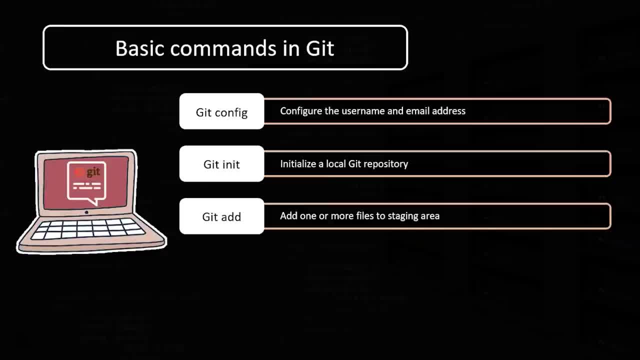 a individual file. so what will really happen? that all those files will be added to the staging area. now why these files are adding to the staging area: so that at any moment of time when you run the git commit command, these files will be picked up from the staging area. 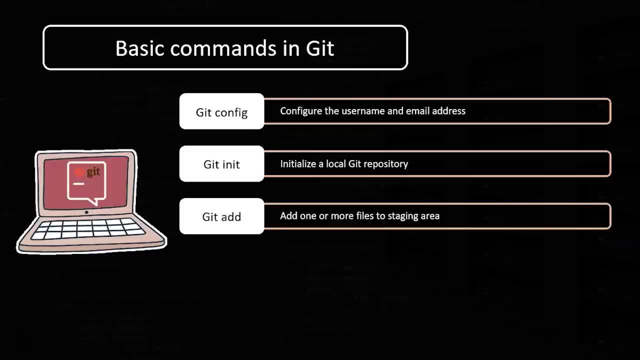 and will be preserved permanently into the git repository. so when you do git add command it moves the files from your working copy to the staging area and it will remain there itself unless and until you don't do any kind of git commit command further, so that these files from staging area will be permanently written off. 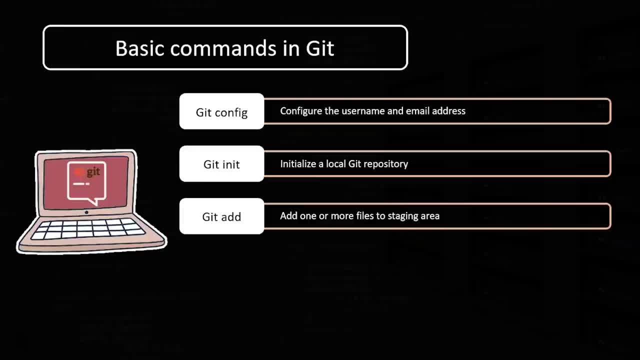 into the local repository. so it's a very important part that you run git add command before running any kind of git commit command. now, git commit command will only pick up those files which is present in the staging area. so if you have been modifications to 200 files or 20, 30, those kind of files. 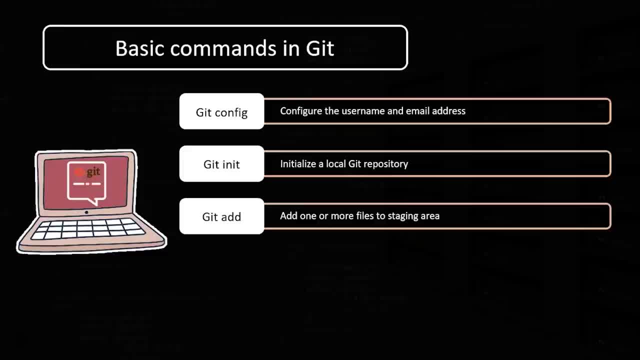 there. if you do the git add command only for five six files, so only those five six files will be taken care in case of a particular commit. so you need to make sure that you select the desired amount of files before doing any kind of git commit activity. 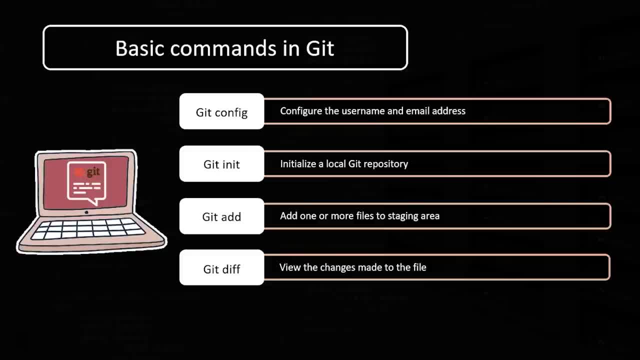 right now. next command which we have here is git diff command. now git diff command is a kind of base tool which we have here which really helps us to understand that how we can check the difference between two files and in fact, this git diff command can also be. 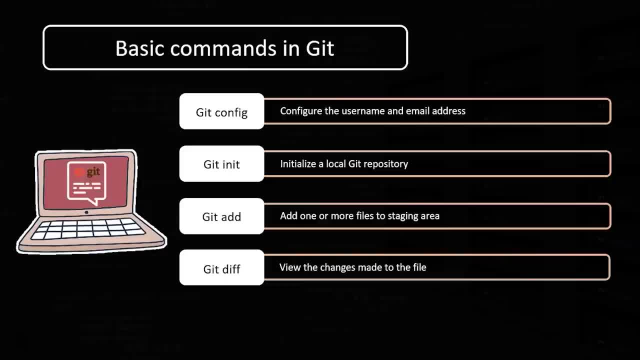 used to see the difference between two different branches also. so if you feel that if you have done some changes to the file, to a specific content here now, if you want to see the difference between your particular head revision number and whatever the modifications do you have done right now, so in that, 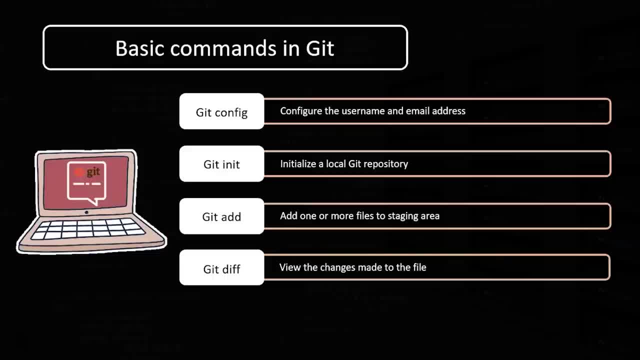 situation. you can run git diff command. it will let you know that, what the different kind of changes and modifications you have done. so if, at any moment of time, before doing any kind of commits, you want to do some kind of review, you want to see that what? 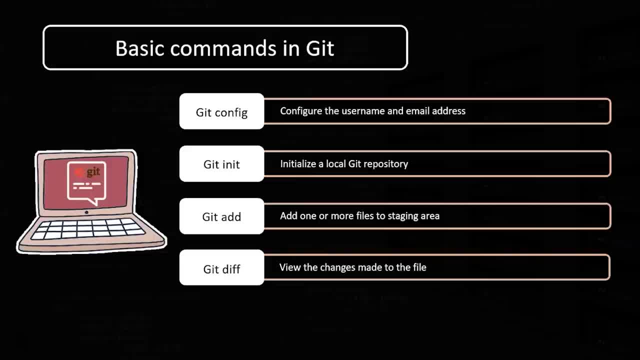 different changes you have done so. in that case, you can go for the git diff command. so git diff command used to see the content, the difference or the modifications which you have done recently to the specific file. right and the last one, we have already discussed the git commit command, which 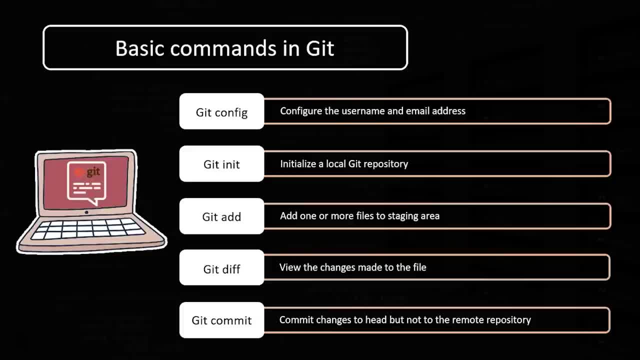 commits, the changes to the head revision number and this commits are something which is stored locally and you will not be doing the direct commits to the remote repository. so commit is something which is done into your local repository only. but yes, this is the last stage of doing a modifications here once the commit is. 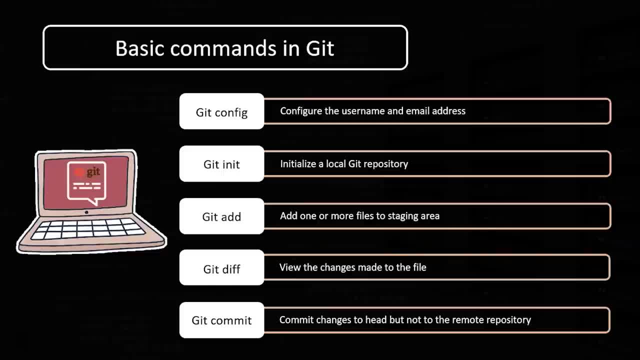 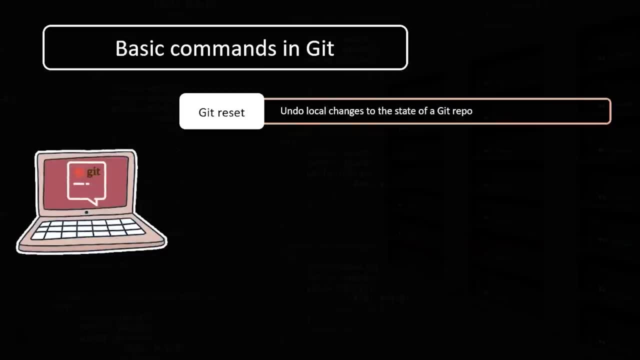 done, it will directly modify your history, your git repository history there, and the changes will be permanently preserved into the repository. so git command is primarily used for permanently preserving the changes into your local repository, right? so these were some of the commands there. now there are some further commands also. 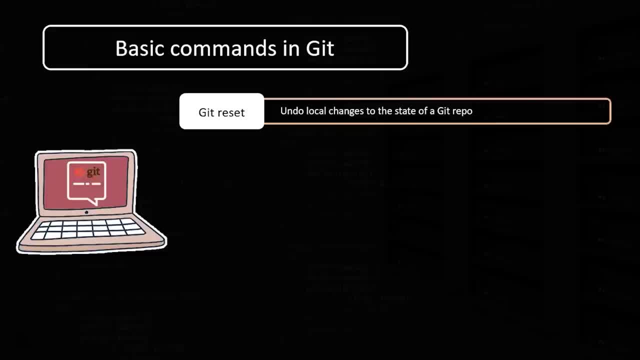 let's discuss about them now. next command is git reset command. at any moment of time you want to do some undo activity for some local changes done to your local repository, into your git repository. in that case we can use the git reset command. then next command is git status. now git status command will. 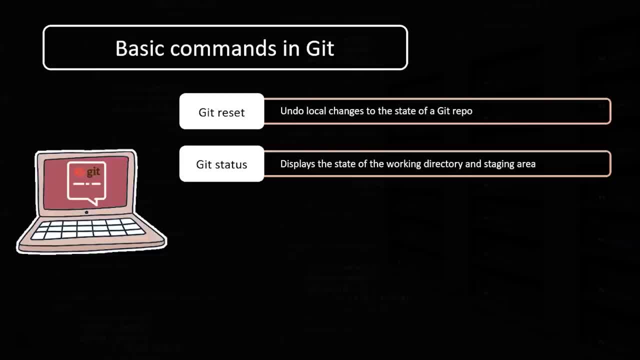 show you the state of the working directory and the staging area. so both these area will be shown when you run the git status command. if you have done any kind of modifications to the working area, that will also be visible to you, and if you add some files to the staging area, that also will be displayed using 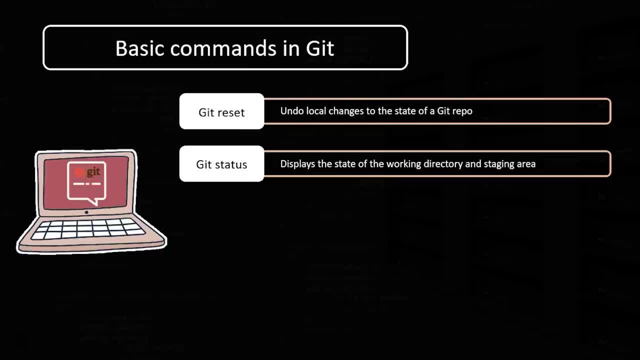 the git status command. so git status command is very important because ultimately it let us know that how the different things and then how the different files are modified over time. here, right, the next thing is git merge. here now, git merge is a very specific command which is used to move the changes from one branch to another. now 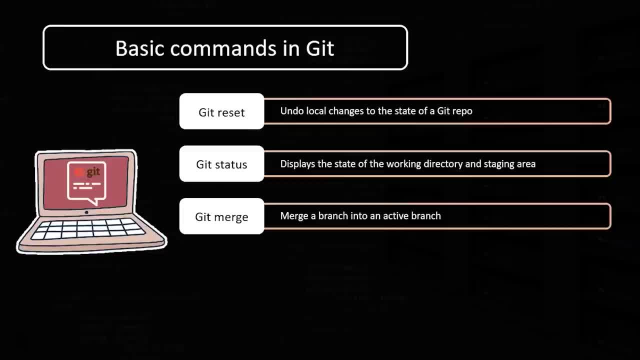 at any moment of time if you feel that you are working on some other branch, like develop branch or some other feature branch, and you want to move the changes from this feature branch to the master branch, so in that case you don't have to do the commits all together again in the master branch, all you can. 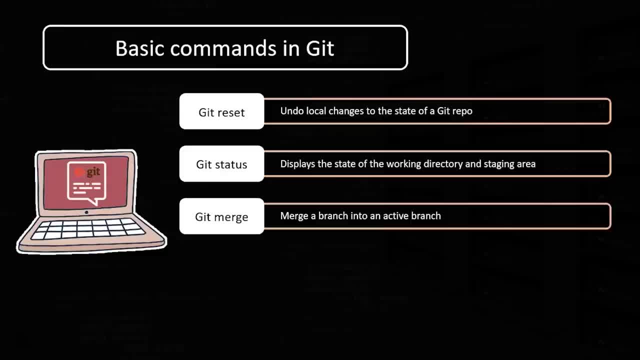 do is that you can go to the master branch and trigger the merge activity. so this merge activity will check what is the difference between the two branches and whatever commits is missed out it will also be synced back into the master branch. so git merge actively helps us to move the changes from one branch to 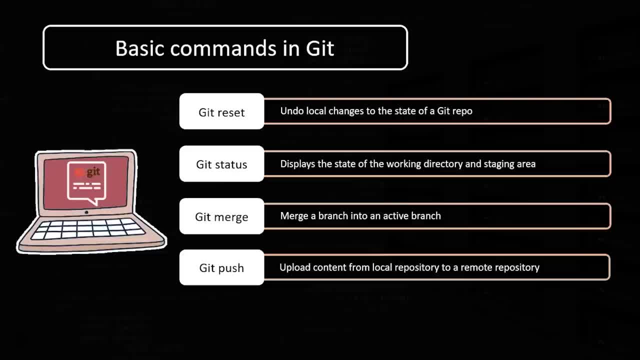 another one. next one is the git push command. here now, git push command will eventually help you to move the changes from your local, to move the different changes from your local repository to the remote repository. now, in this case, what happens? that if you are working in offline mode, if you have done some, 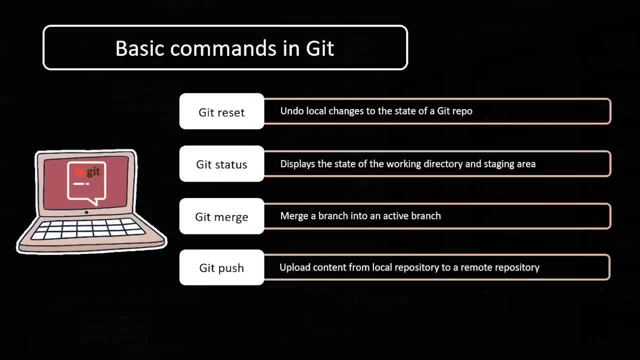 couple of commits. now git push will help you to sync those commits back to the shared, to the remote repository. now these remote repository can be github, bitbucket or gitlab. that is a different story but, yes, all your changes will be synced or will be moved from your local repository to the remote repository. 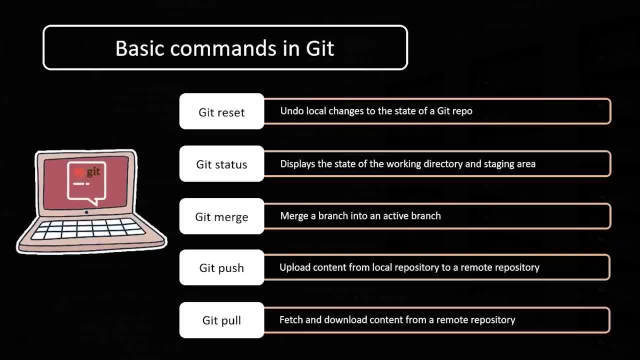 right, and the last one is a git pull. git pull is an activity of push here. now you might have seen that some other developers are also doing some check-ins or some push activity to the remote repository. now, if you still work on an old version of your source code, it may cause a lot of. 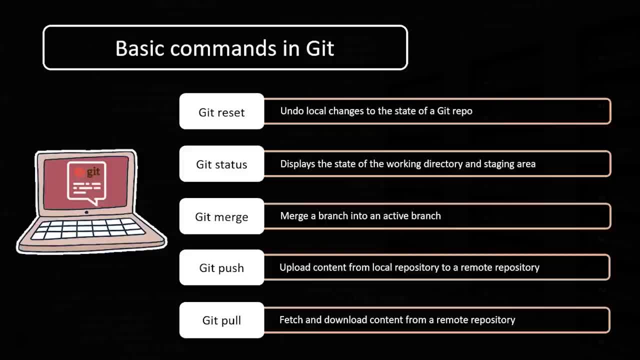 problem for you. so at frequent intervals you may have to pull the changes or you may have to download some changes from the particular network or from the remote repository. once that is done, you will be able to see that those particular changes will be pulled down and you will be pretty much able to do the you will be able to. 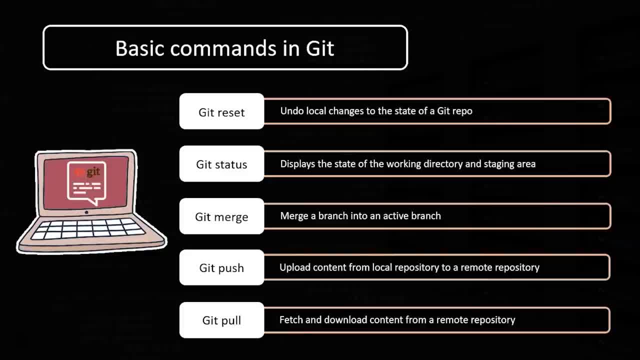 fetch and download the changes from the remote repository to your local repository here. so this is an activity which really helps us to understand that how we can pull some changes from the remote repository to your local repository so that you can have the latest source code which might be pushed. 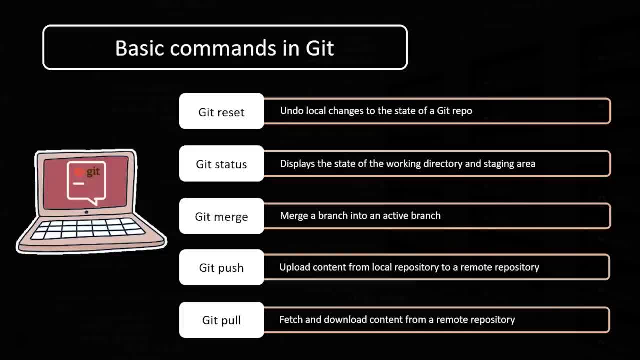 by some other developers or by some other collaborators, so that you can always work on the latest source code into your local system. so this is again a mechanism in which we are trying to see that what are the different git commands we can explore and we can utilize here? 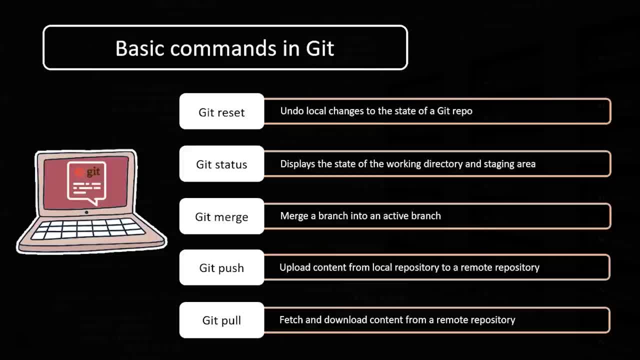 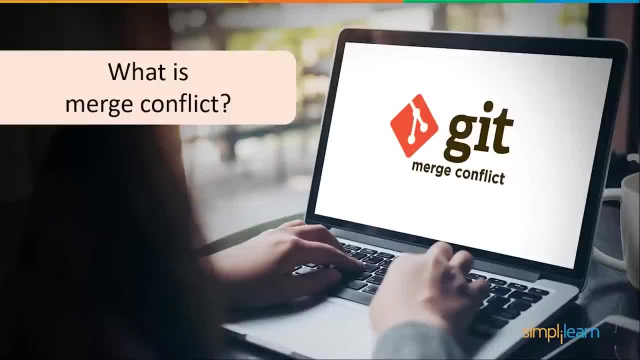 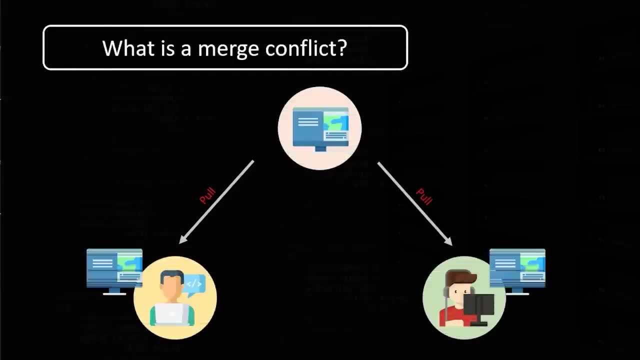 to interact with the git repository. so this was some of the basic commands which we can use for managing the git repositories here. now let's talk about that. what exactly is a merge conflicts? now, merge conflict is some thing which gets originated the moment we do some kind of merging activity. now, 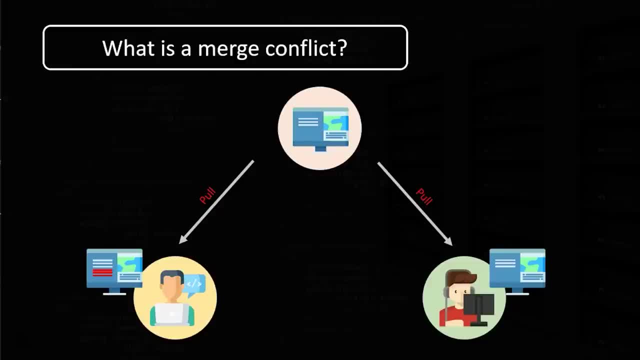 merging is an process in which we move some source code from one branch to another. now all the developers cannot work on the same piece of branch there. so what really happens? that in that situation all the developers mainly work on some couple of branches and then they all collaborate to some other branch or 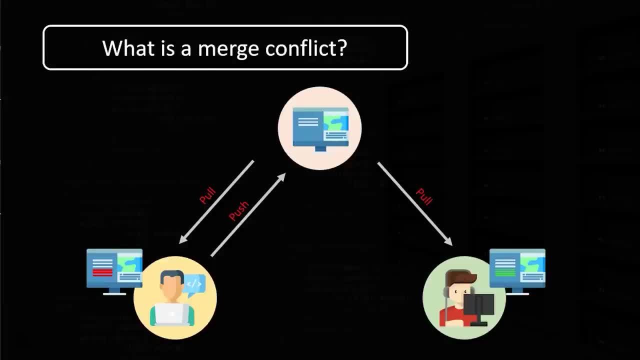 different developers try to push their changes from the local repository to the remote repository, so in all these situations, the source code gets moved from one location to another. now what happens in? as per this diagram, we have a remote repository over here. now all we are trying to do is that we are trying. 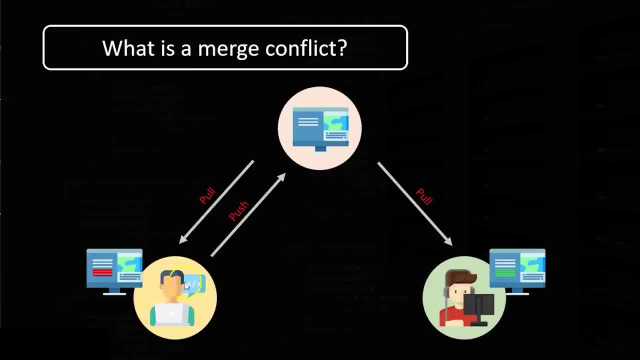 to push some source code over here from a particular developer here. now he is doing the pull and push activity and this another developer is there who is also doing the pull activity here. so merge conflicts basically happens then, for example, this particular developer A is trying to do some push right, so that 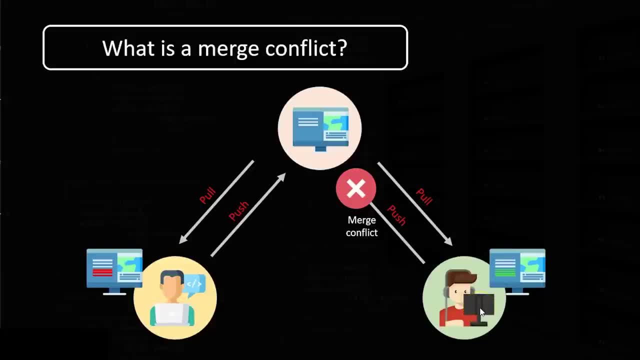 push is almost done here and when the particular developer V is trying to push the particular results or try to push its own content to the remote repository, he got a merge conflict which means that his particular developer B merge activity is cancelled, is deferred here. now it could be a possibility because of 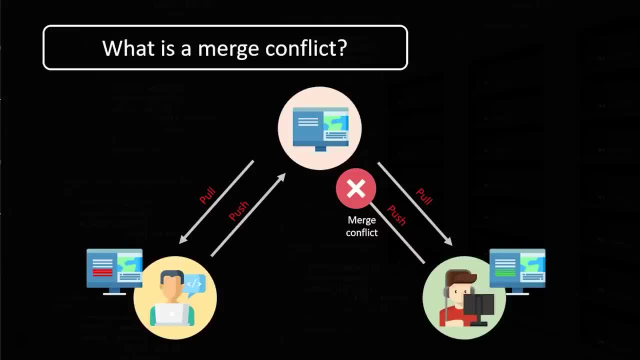 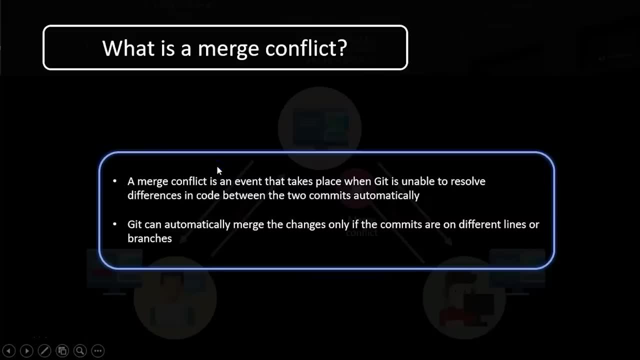 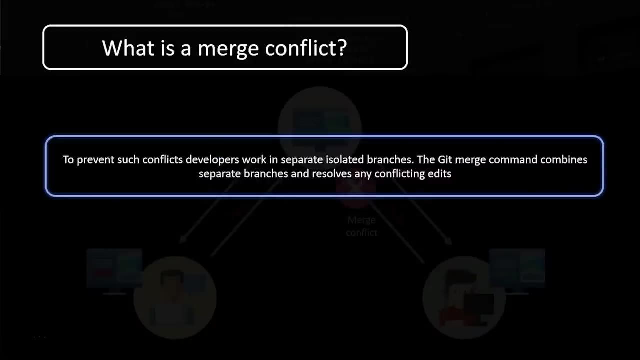 the changes on the difference on the two piece of source code, which means that the source code there. so let's talk about that now. in order to prevent such kind of conflicts, developers usually provided with the isolated branches so that they can work on their branches and once the development is done, they can do a single. 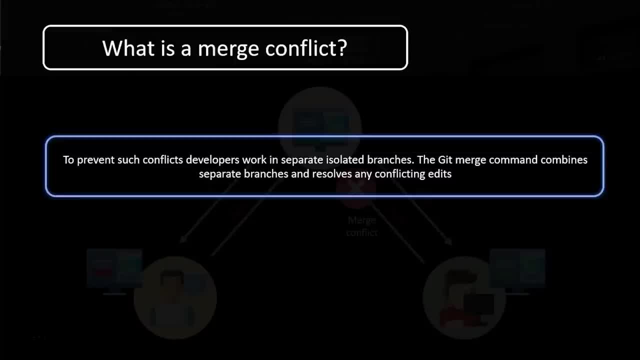 merge and they can sync their changes into a single branch. so the git merge command combines separate branches and resolves any conflicting edits over there. so once the developers are done with the specific changes, with the modifications to the source code, later on they can combine those things, they can work on these components and they can resolve all these. 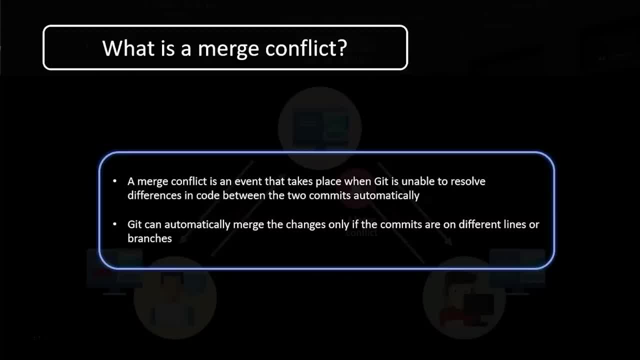 conflicting modifications. right, so a merge conflict is an event that takes place when git is unable to resolve the differences in the source code between the two commits automatically. normally, the git is having the capability to understand that. okay, these are the two different piece of source code which is getting pushed to a remote repository, but in any case it does not. 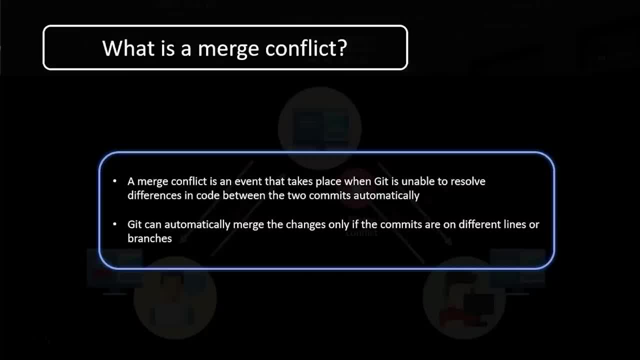 happens automatically. there is any kind of conflict which arises over there and git is not able to take any kind of decisions. so in that situation we will be able to get a merge conflict. now it could be a possibility that one merge can happen successfully. then the next merge will be cancelled and will be 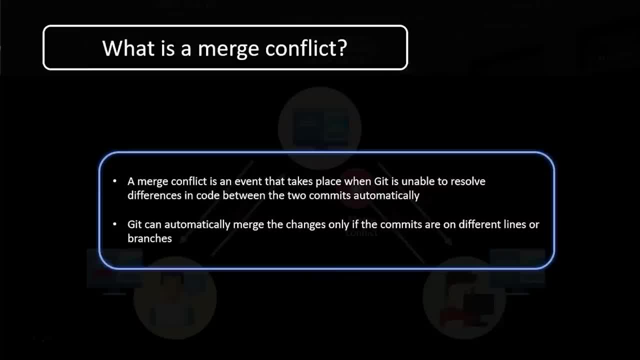 deferred due to this. merge conflicts. so git can automatically merge the changes only if the commits are on different lines or the branches here. so if at any moment of time you are diverting from the process, you are having some different lines of source code, so that is where the merge. 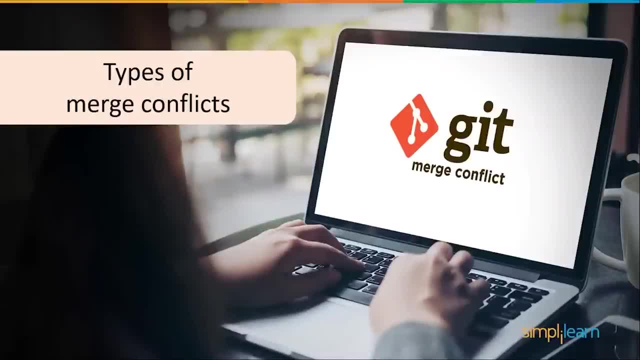 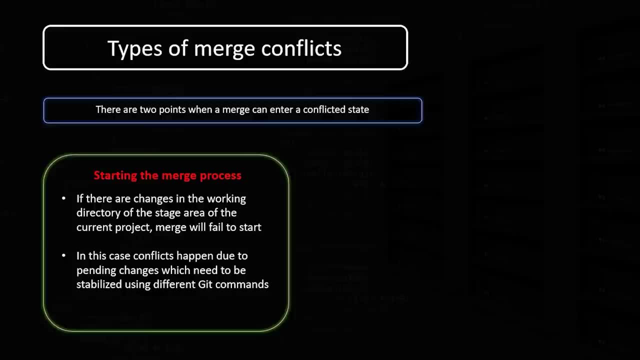 conflicts comes into the picture. now, what are the different kind of merge conflicts which we normally face? the main types of merge conflict is: first of all, there are two points where we can say that a merge can happen or can come into a conflicted state. the very first one is the started the merge. 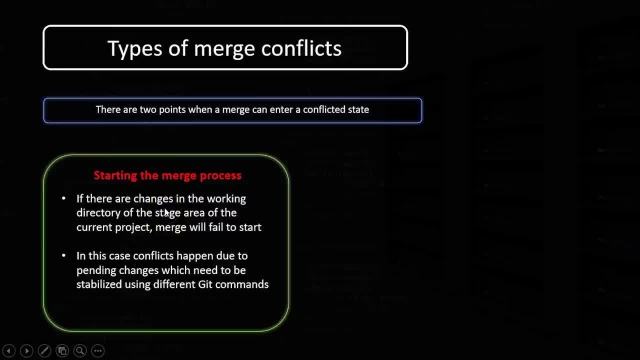 process. now. if at any moment of time there are changes in the working area or working directory and we are moving, or these changes are getting moved to the particular working area of the stage area of the current project, so during the merge activity itself the particular merge will fail because there are some. 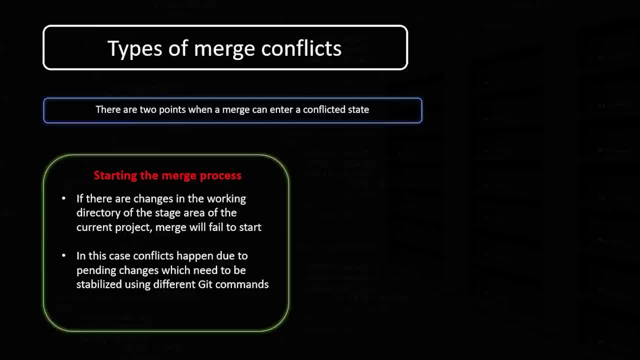 changes or there are some kind of modifications right now present over here in the working area. so in this case conflicts happen due to pending changes. now, for instance, you have done some modification to the changes. now you were planning to do the commit, but before that you felt 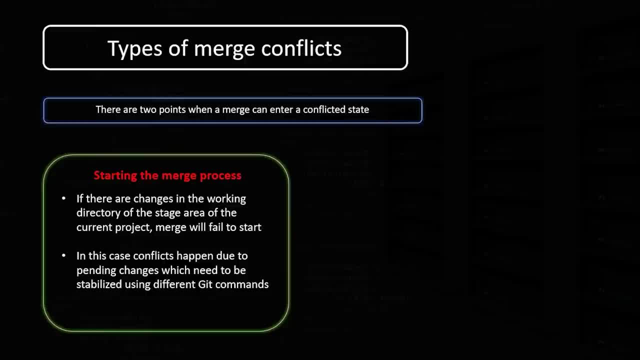 that I want to do some kind of merge now, since there are some pending changes which is available there into your working area. so what will happen? that your merge will definitely will there itself. so before even starting, before even in initializing the merge, as in particular pre-check, your merge activity will fail there itself. so in 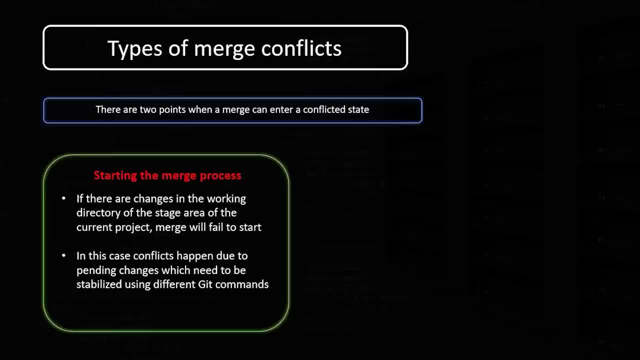 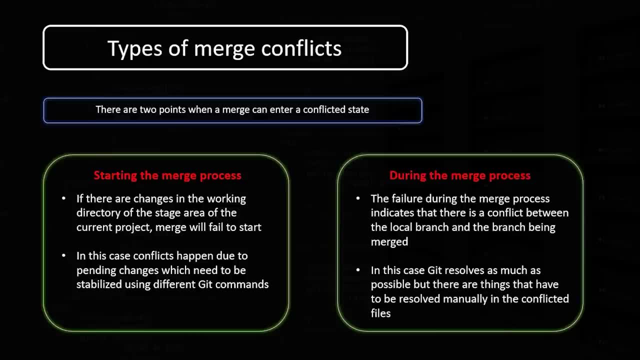 that situation you have to either remove those pending changes or you have to resolve those pending changes before even going for the merge activity. second, during the merge process. definitely if you are getting some conflict, so the merge conflicts gets originated. so the failure during the merge process indicates that there is an conflict between your local branch and the branch. 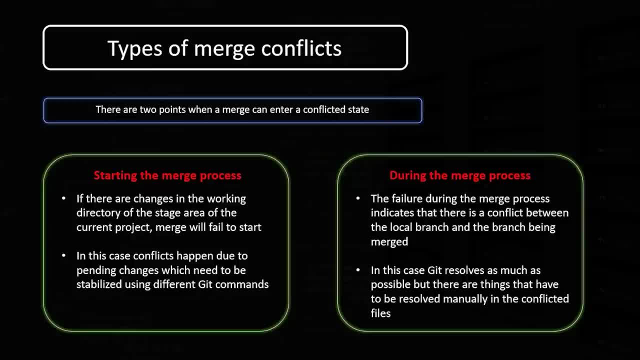 being merged right. so you're trying to move the changes from one branch to another. so it means that there are some particular conflicts which is coming up in the particular branch in which you are trying to do the merge. so in this case git resolves as much as possible. so if there is any kind of difference in the 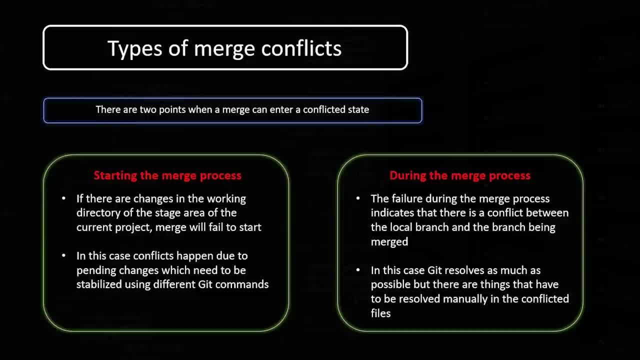 source code in the commits and the different line of source code there. so git automatically try to resolve it as much as possible, but at any moment of time it's not able to do, it's not able to manage, in that a particular human interruption is required so that we can merge or we can. 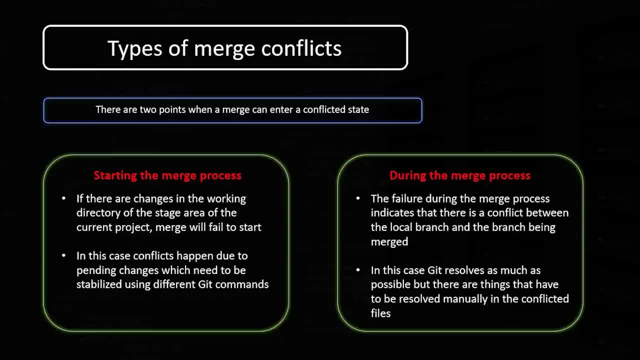 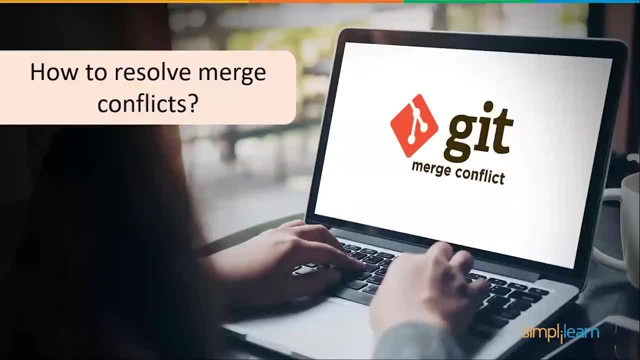 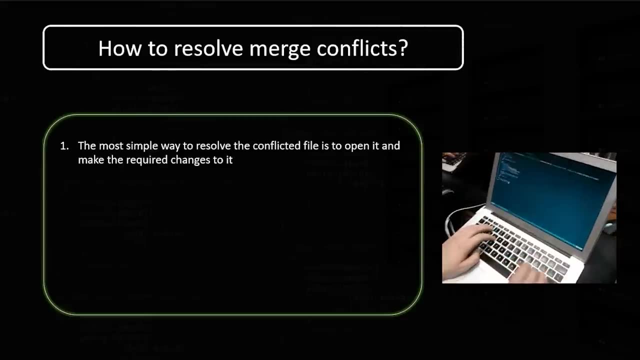 resolve this particular conflicts manually there. so these are the two types of situations in which a particular merge can enter a particular conflicted area. now, how to resolve these merge conflicts? now, what happens that, in order to resolve this merge conflicts, the simple way to do this is that we open. 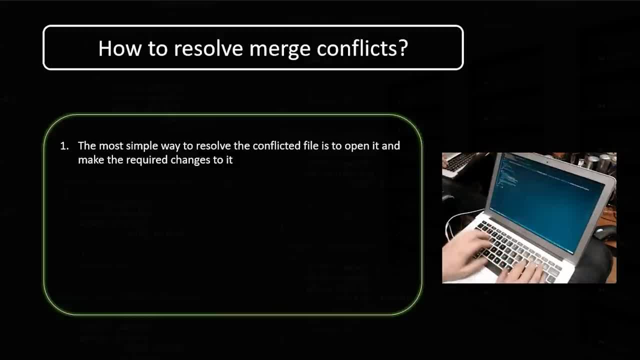 the file which is in conflicted status. now, once that is done, you do the required changes. whatever source code you feel you want to proceed, you will select that source code, you will use that source code and once the addition or editing of the file is done, so what? 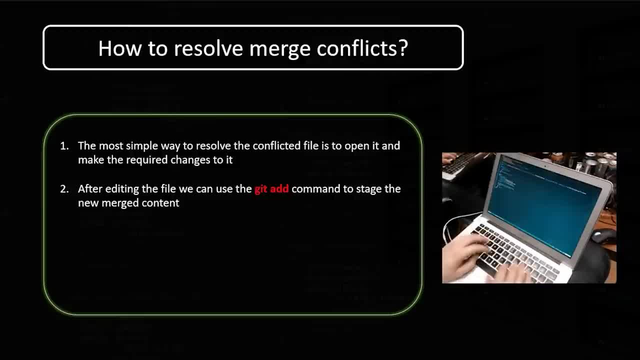 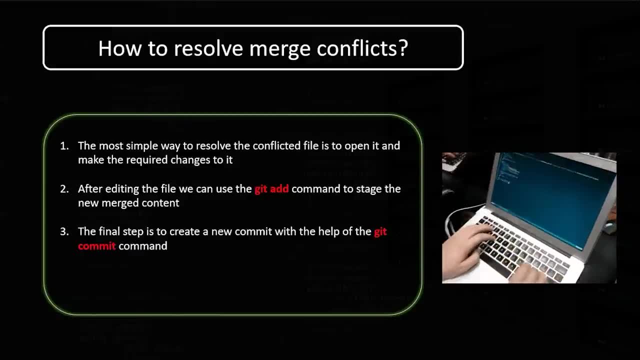 you can do is that you can run the pretty much straightforward command called git add to add that file to the staging area, and then what you can do is that you can do the git commit activity so that the particular merge conflicts can be resolved and you will be able to see a merge here. now this is a something which is 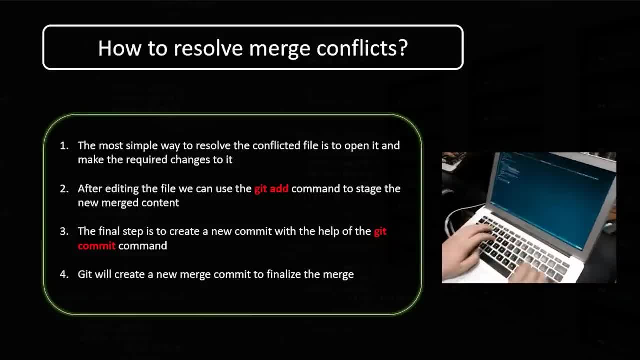 known as one of the best approach for resolving the merge conflicts because even if it comes up, if git is not able to handle it automatically and it requires for you to manage it manually here. so definitely in that situation we have to open the source, we have to select that which portion of source code. 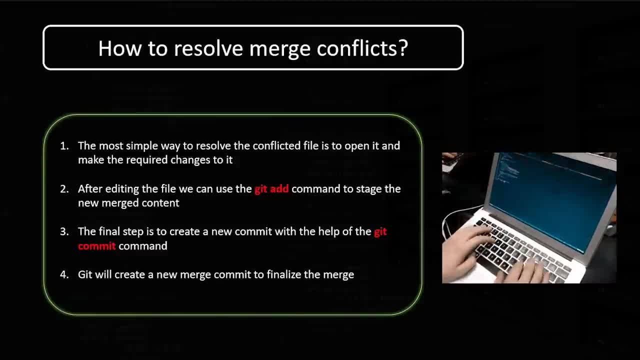 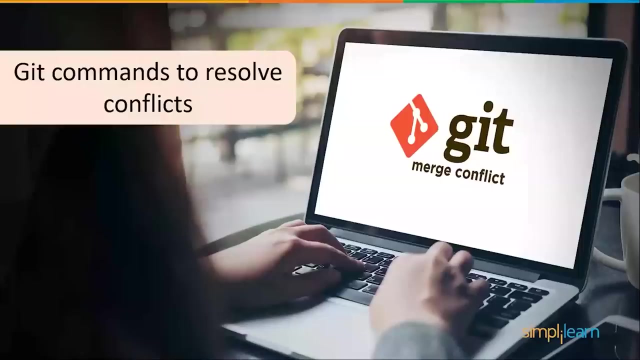 we want to keep do the modifications manually and then follow the traditional approach to control. we use git add to perform a custom commit. so git add and git commit command- you will be doing their in that situation to have a particular final merge executed altogether. so this is the steps which we can follow to perform a custom to. 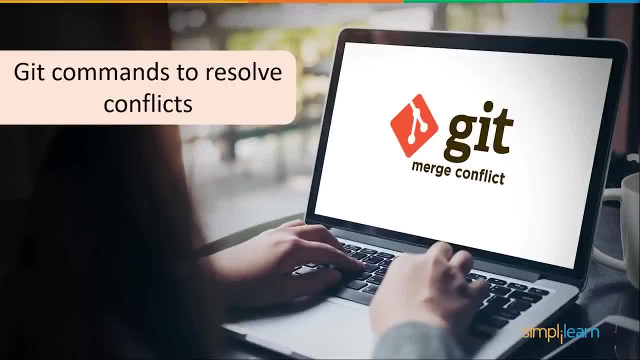 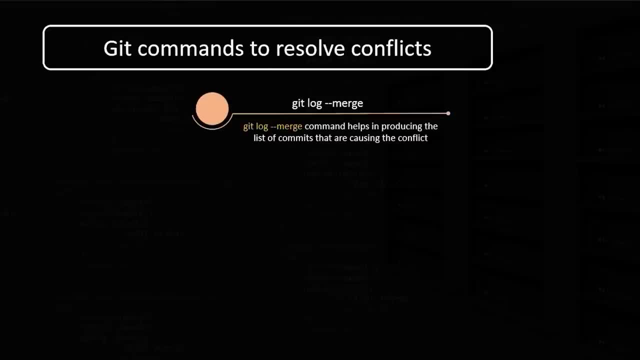 resolve a particular custom merge conflicts over here Right now. the various git commands which we can use to resolve the conflicts here, now commits that are causing the particular conflict here. if at any moment of time your merges fail down and you want to see that what are the different commits which is causing the 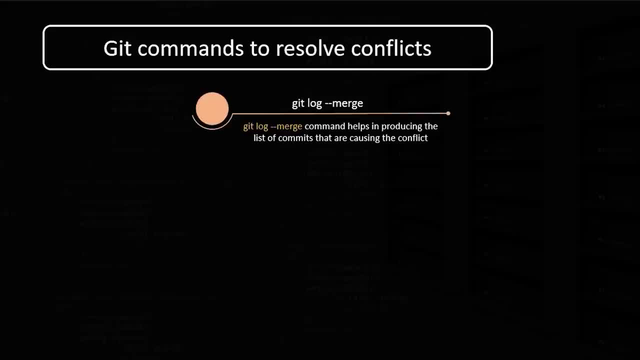 issue here? probably you might be, you know, ignoring some commits which is not that much important, or you can manually override the content so that those conflicts data can also be added and whatever the changes you are trying to add, that also should be modified. second command: git diff command. you can always use the to check the difference between the. 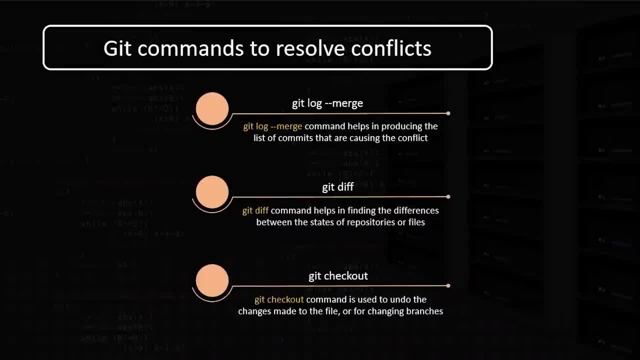 particular files between the repository. git checkout is something which you can use to particular checkout a file, so that if you want to check out the latest content of a specific file or a folder, so in that case you can make use of this git checkout command here. so git checkout command will definitely help you to understand that how we can go. 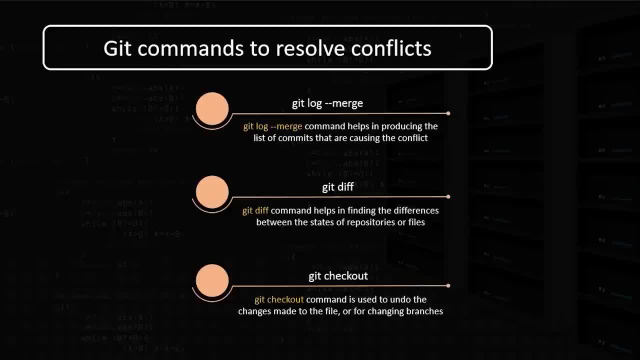 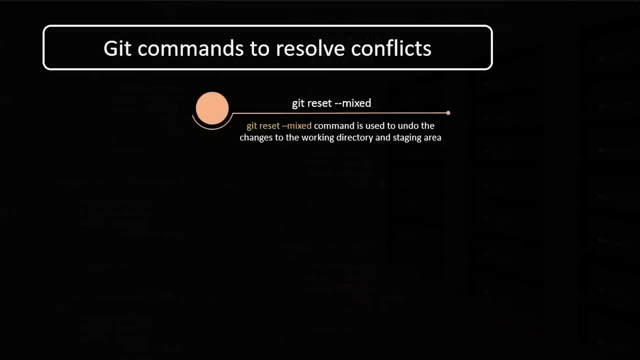 for or how we can do the checkout of this particular repository or a particular file here. right, so then we have a command called git reset hyphen hyphen mixed. so git reset hyphen hyphen mix is then command to undo the changes of to the working directory and whatever the particular changes you have. 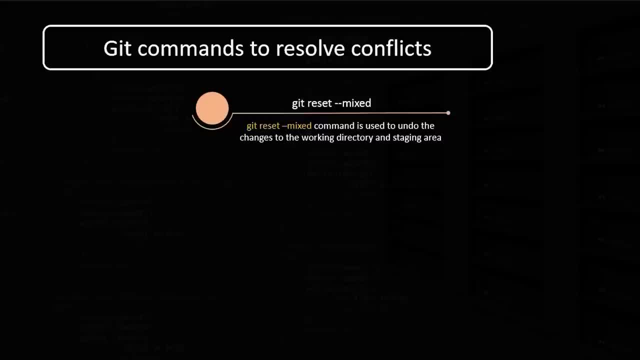 so that will be undo there and it will be able to do the undo changes to the working area and the staging area here now. then we have git merge hyphen hyphen award, which will be used in order to exit the merge program, and then we have git merge hyphen hyphen award. 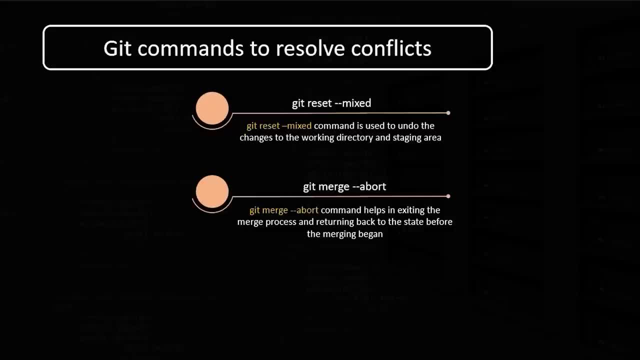 now the next thing you can use to do is to go to open git and click on exit the merge process and return back to the state before the merging begin. if you not able to resolve the merge conflicts manually also, so in that situation we will be aborting the merge situation. 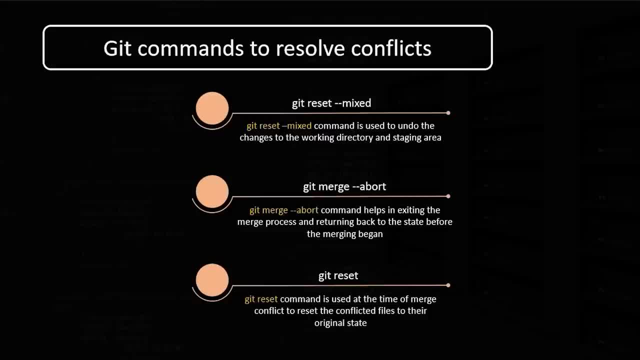 or a git merge over here and the last one is git reset. so git reset command is used at and time to of merge conflicts, to reset the conflicted file so that what we can happen, that we can go back to the previous situation before even starting, or the state before you. 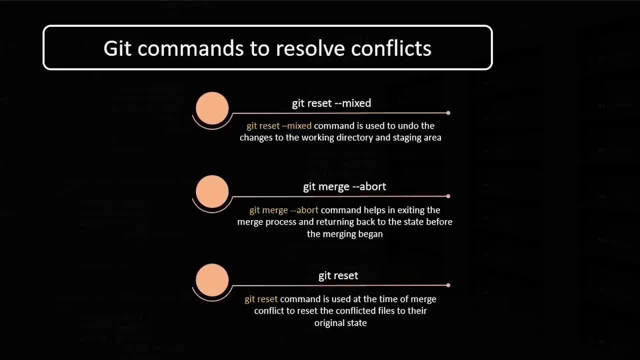 before the merge activity was started there. so git reset will eventually help me to reset all the files which is in conflicted area, and our latest files will be checked out and will be replaced. so these are some couple of commands which we can actually use in order to resolve the merge. 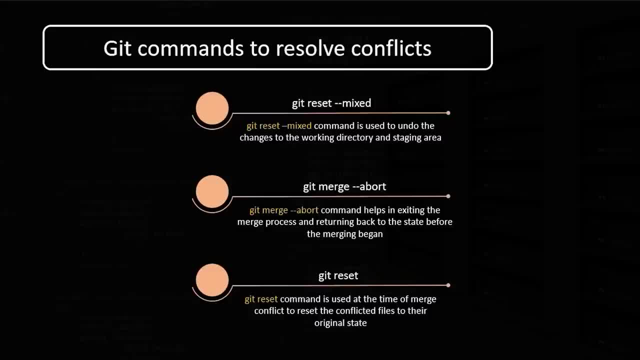 conflicts into a git repository. now that was something which we were trying to understand, that what exactly the git merge was there and how the git merge originated and how they get particular merge conflicts gets created and how we can resolve it. now let's go for a proper demo. 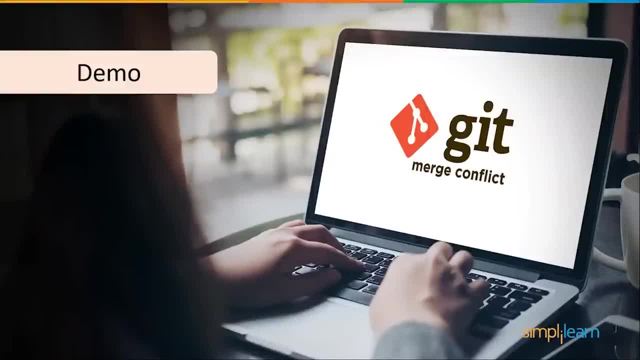 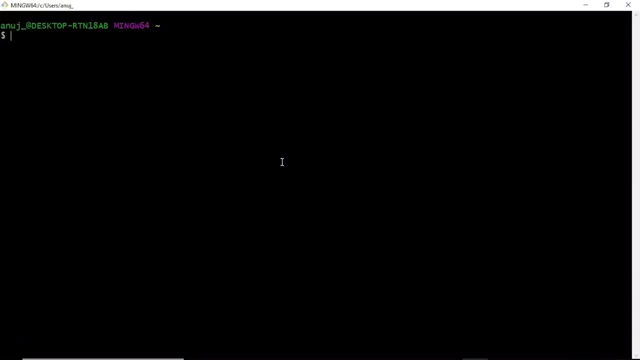 on this one so that we can understand it properly, that how exactly git merge conflicts really work and how we can resolve it. now. this is the git bash which we have installed to run some git commands. now in this one, first of all, i'm going to create two repositories, so i'm going to run the command. 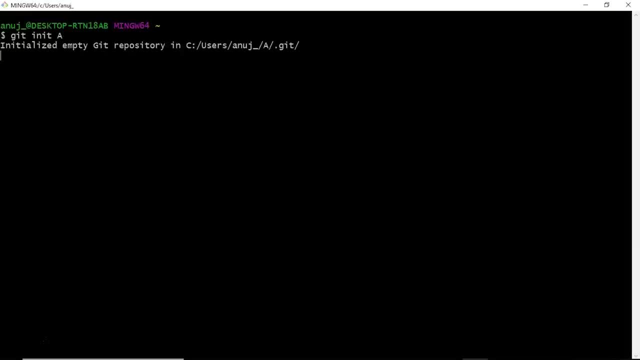 called git init a. that will initially a repository. git init b- that will initialize a b repository here. so two repository. i have got a and b now in basis a. what i'm going to do is that i'm going to add the remote. so git remote, add origin. 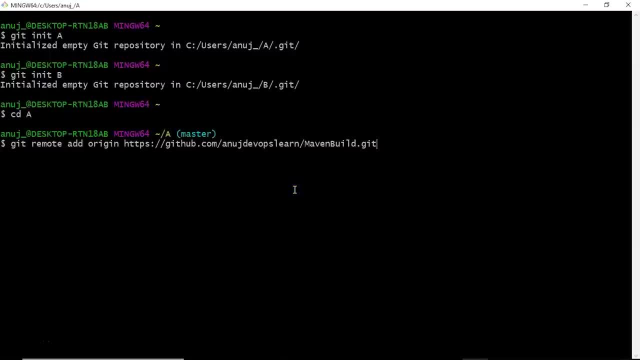 so i'm just trying to add the origin over here. so the origin over here in this one is the maven build. so this is a repository which i have got into my github account. the moment you do this, what next you can do is you can do the next step, you can do the next step, you can do the next step. 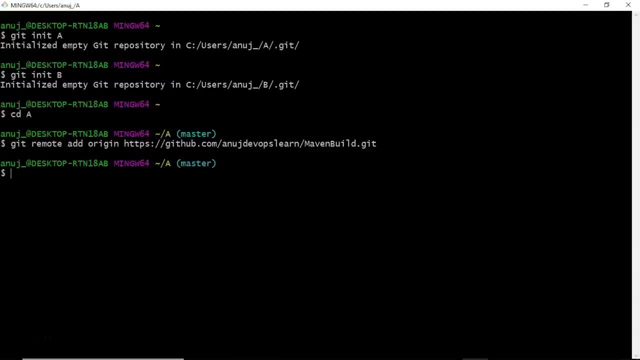 you can do over here is that you can run the particular next git pull command to fetch the latest updates here. right, so next move to the particular next command here. now, when you do this, what will happen? that all the changes which is present in the remote repository. 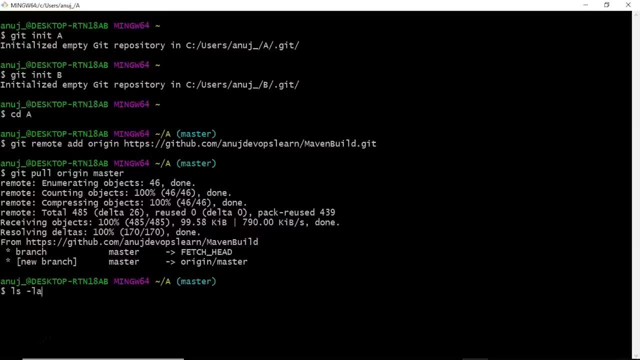 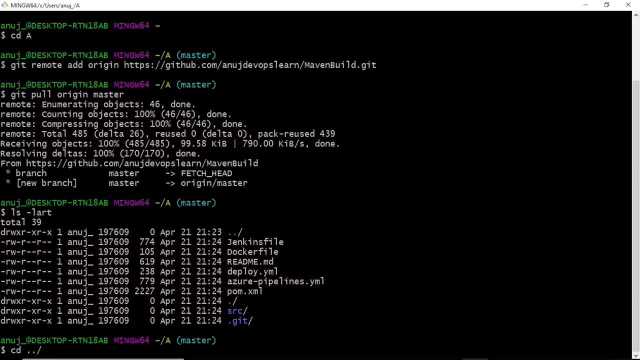 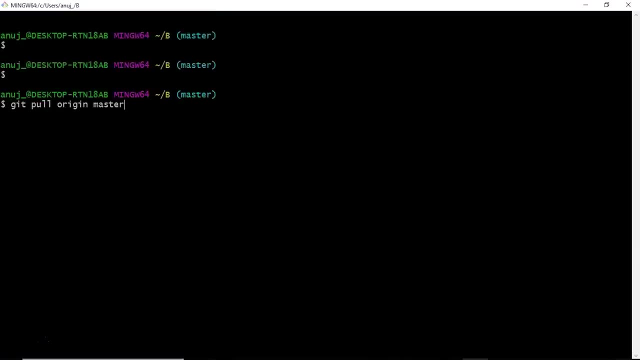 or central repository will be available here also, right, so you will be able to see some couple of files all together here. now the same activity you have to do in the particular b directory also or in the particular b repository also, so you have to add the url, the remote url, here. 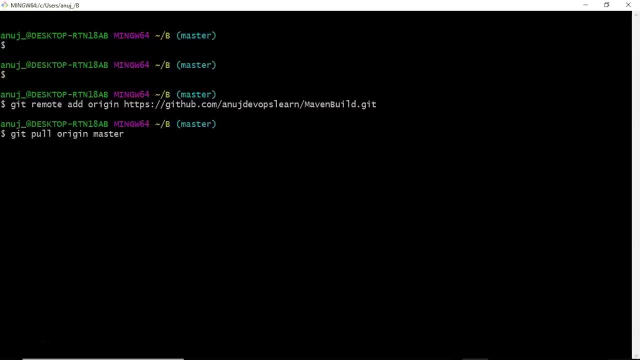 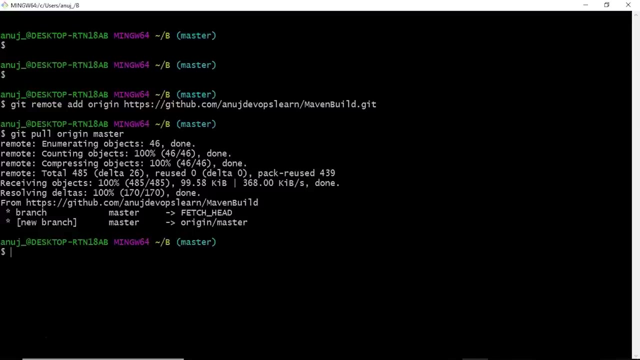 and in this case also we are trying to fetch the particular values here. now what will happen? that we will be doing some modification in the particular a repository and then we will be pushing that change to the remote repository and then through the b when we try to push the changes. so in that situation we will try to see that what really 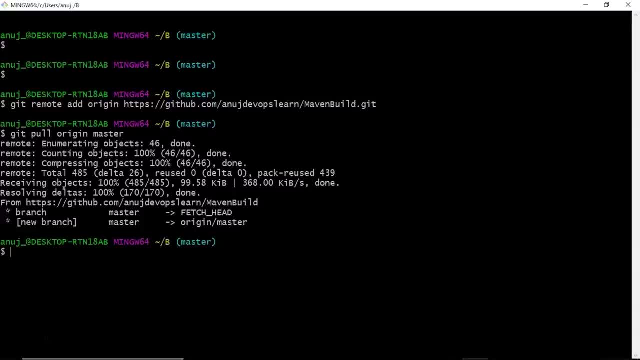 happens, do we really get the merge conflicts? because both of them, although is trying to do the changes to the central repository, but these two repository represents two different local repositories, probably in two different developers machines over here. so that's what we are trying to replicate here. so i'm going back to the a directory here so that i would be able to do some changes. 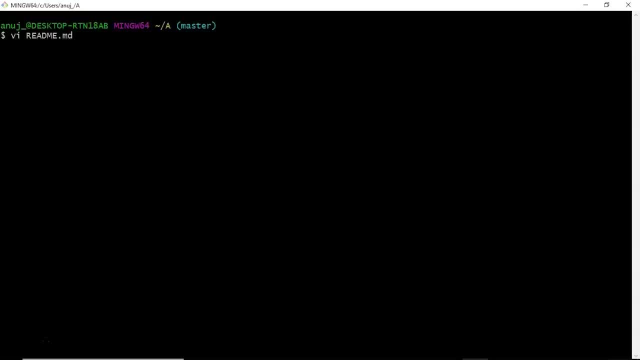 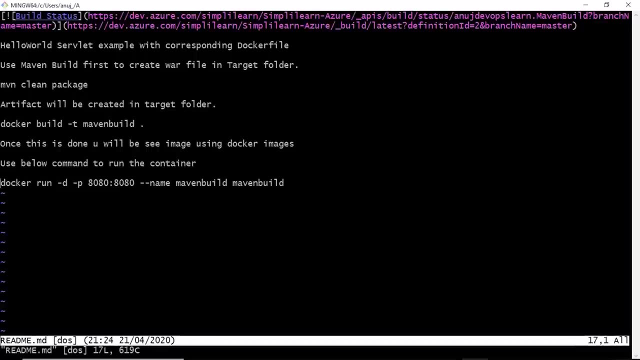 all together. so i'm just opening readmemd file here. so pretty much i'm just trying to add some particular changes over here to this particular file. so this is what we are trying to do here now let me add some particular additional and a particular new line over here in the file. 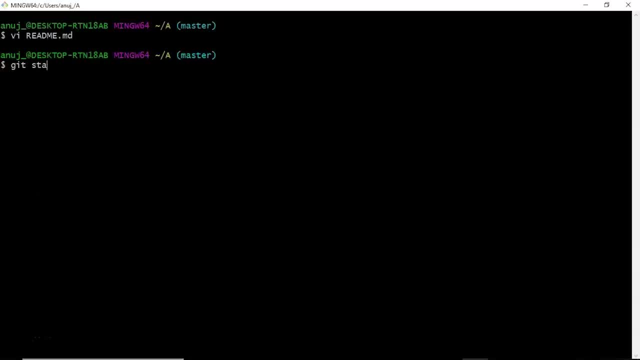 and then save the content. now, once this is done, i will be able to see that, yes, there is a particular change which is done all together here. so you will be running git add command and then git commit command to save the commits all together. so we are giving a particular commit here so that we will be able to identify that this is. 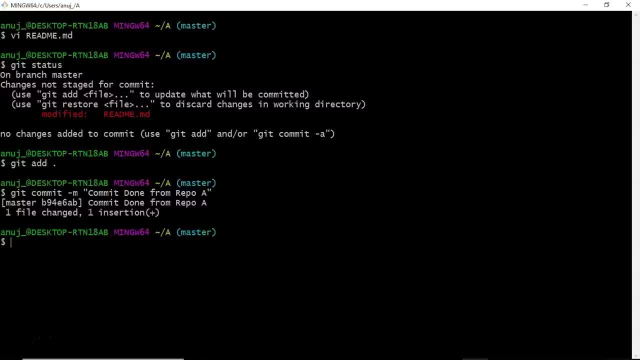 something which we have committed from repo a. now, once this is done, i will be doing the push activity so that i can push these changes to the particular remote or the central repository here. so exactly what we did over here so far. we have a particular novo in the center of the repository here. so over here we see that this is, for example, 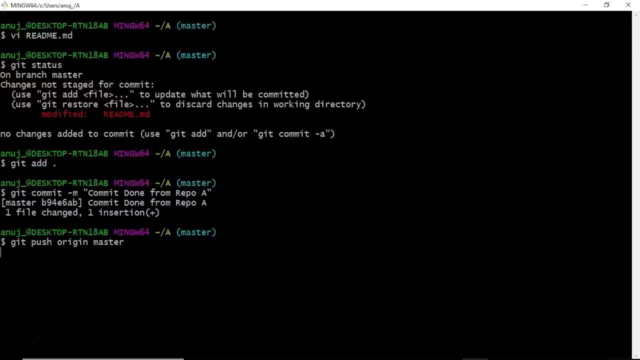 downloaded remote repository in a repository A and then we are doing some changes, some modifications, and once those modifications are done we are pretty much changing or putting up that new commit all together to the github repository. so this is what we are trying to do so far over here in this one. so 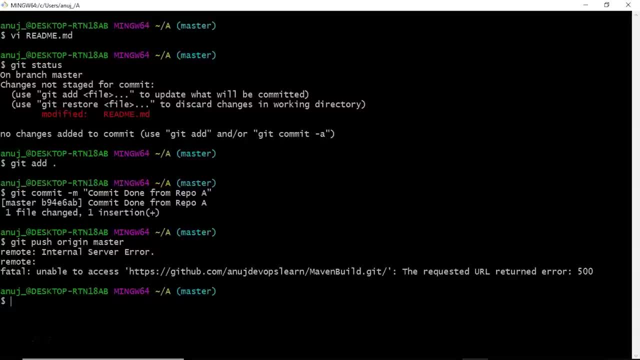 this git push activity will take the particular access right. so when I do the particular push activity here. so if the credentials are saved, then that's fine. otherwise it will ask for the particular user name and password all together here. so that will be asked by the particular activity. 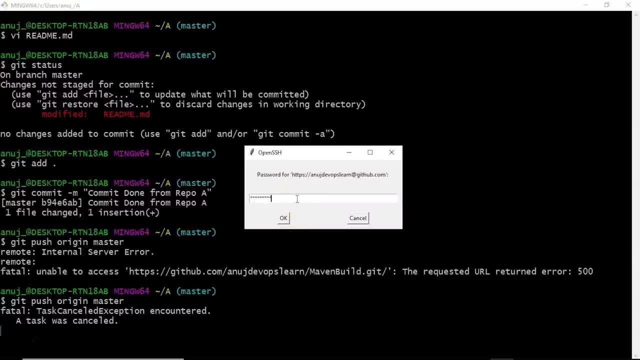 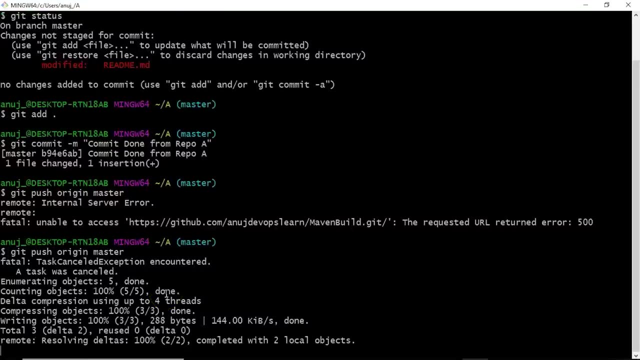 here. so it will ask for the password. so all you have to do is that you have to just share that password and your git push activity should be passed on or should be, you know, done there. and, as you can see, that changes really got moved to the github repository now sometimes, 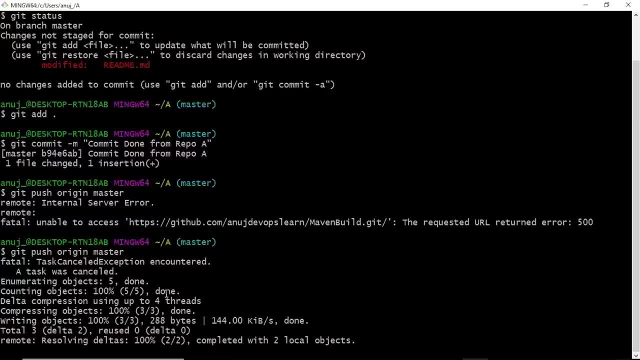 you have to do some changes to the github repository. and sometimes you have to do some changes to the github repository and sometimes the credentials get expired. so you may get some particular message saying that you have to put some password there. a particular interactive window will be open there and you have 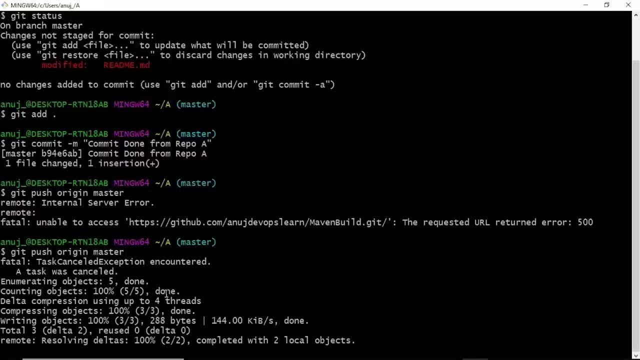 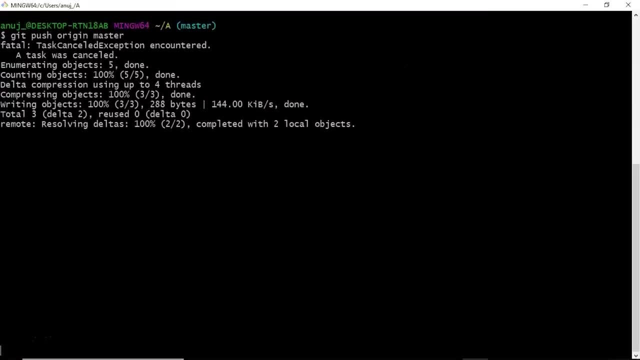 to prompt or you have to provide that password and according to that it will proceed further. right, so this will eventually help you to move the changes into the github repository all together. so all of your changes will be pushed to the github central repository right after some time. it. 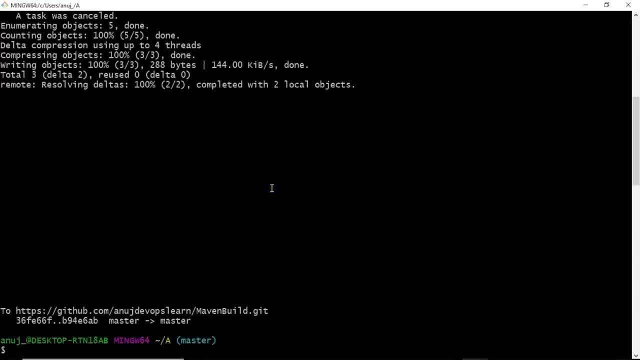 really pushes my comments to the remote repository. it will take some time, depending on the network connectivity and the kind of changes you are trying to upload. so now, since my particular repository is done, so what I can do is that I can further go back to the particular directory here. now, what we 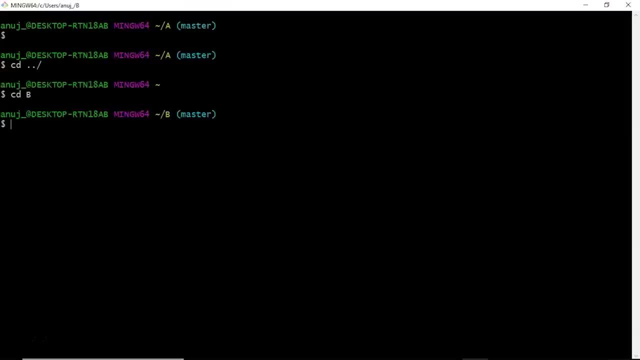 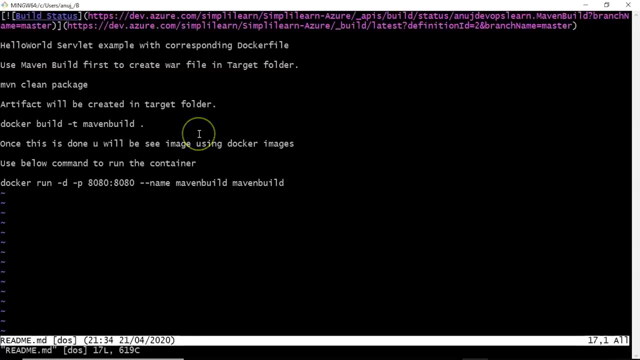 can do is that we can go back to the beat repository over here, and in this case also, I am just trying to do some modifications, so for instance, that I am just trying to do the changes here to the readme file again, of kind of a changes in this one. now, in this case, I am trying to delete this line, the last. 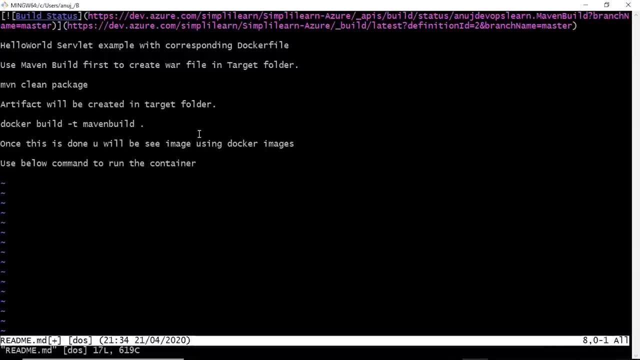 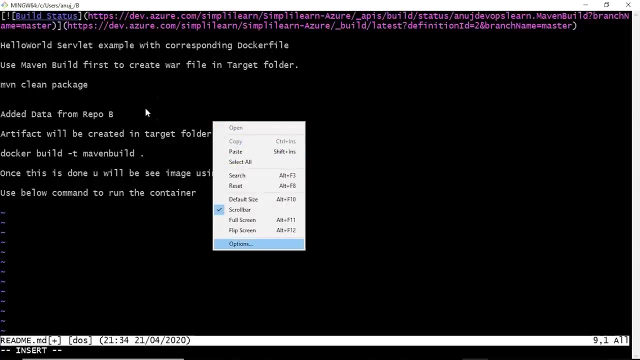 line I am trying to delete here, or a couple of modifications I want to do over here, like added data from repo and then further most I want to have. let me do some arrangement like let me have this data added all together over here or I can add it. 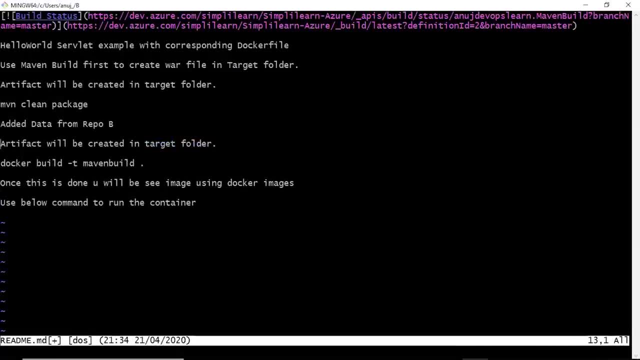 yes, so data is added and this data is removed. so the idea is that we can do different kind of free shuffling of the data up and down so that we can understand that how it really works. so I have shuffled the data, I have removed. so a couple of lines and let's see that how it works. right, so I have even added: 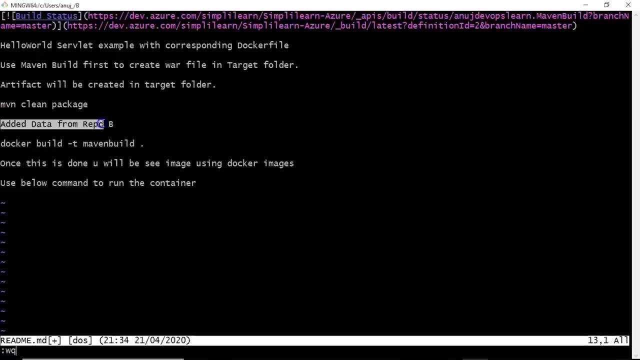 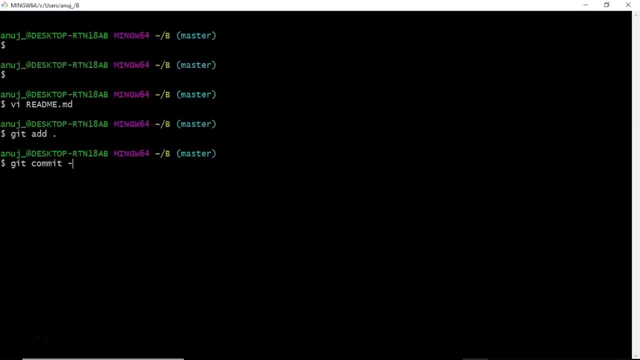 some couple of lines over here. in this new line I have added one line I have removed from the last and this particular line I have shifted five, six line up over here. now let's me save this file and then run the git add command. after this we are going to run the particular commit here saying commit. 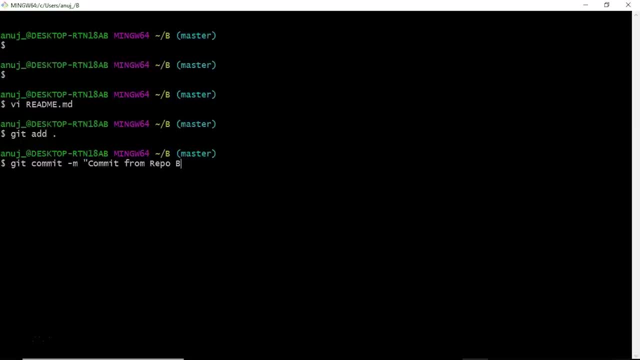 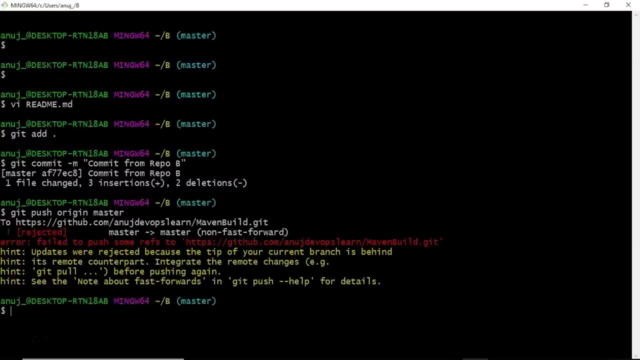 from repo B once commit is done. same activity: pushing it to the remote repository. now let's see what really happens now. when we are trying to push this particular change to the remote repository after the change was pushed from repo a, it will throw an error saying that the particular due to the 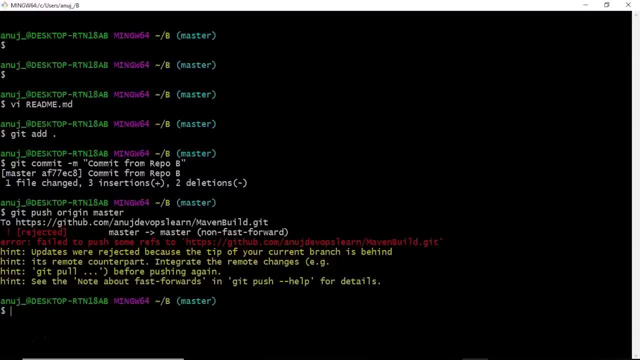 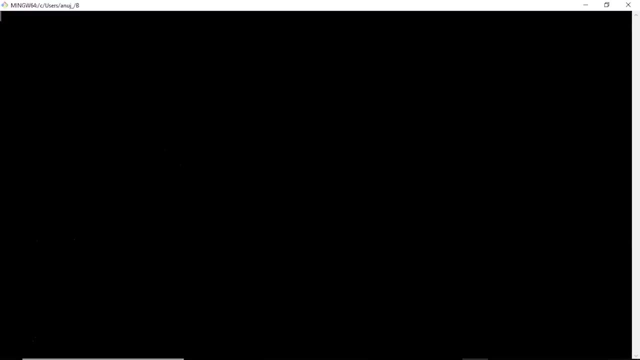 conflicts, the updates are simply rejected here, right? so in this case, what really happens? that, because we are having a different stream of source code in a remote repository and from local repository, you are trying to push some different line of source code. so what next you need to do is that, first of all, 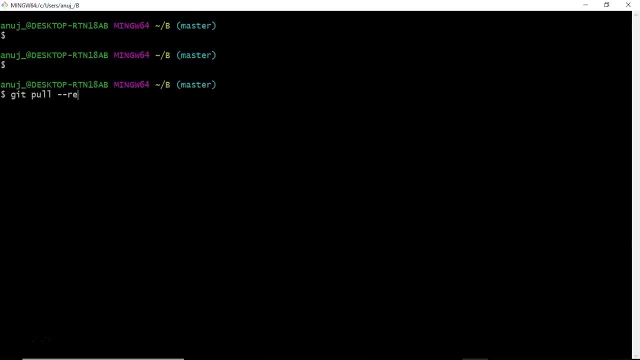 you need to do the activity called git pull hyphen, hyphen reverse origin master. so you're going to pull the changes from the remote repository so that you should be able to get some particular content all together in this particular repo b over here now, the moment you run this. let's wait for this activity. 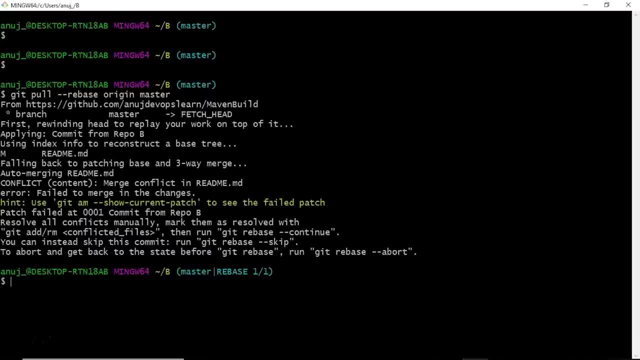 now. once that is done, you will be able to see that you are seeing a message saying that conflicts are there. so first of all you have to resolve this conflicts and then it will be proceed further. you have some couple of options. like you have to resolve the conflicts manually. 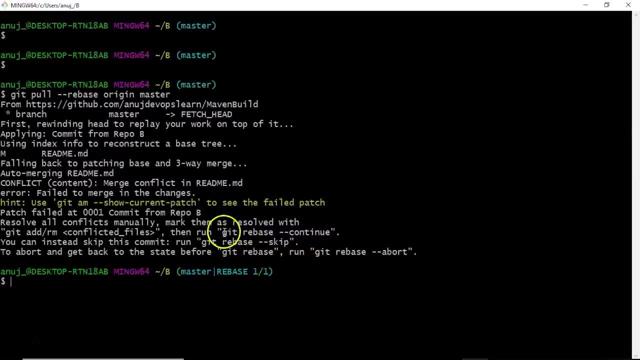 and because git is not able to handle it. otherwise, once the git conflicts is resolved, you can run git reverse, hyphen, hyphen continue. if you want to skip this commit, so you can say git reverse, hyphen, hyphen skip. and if you want to abort the particular, this reverse here. so in that, 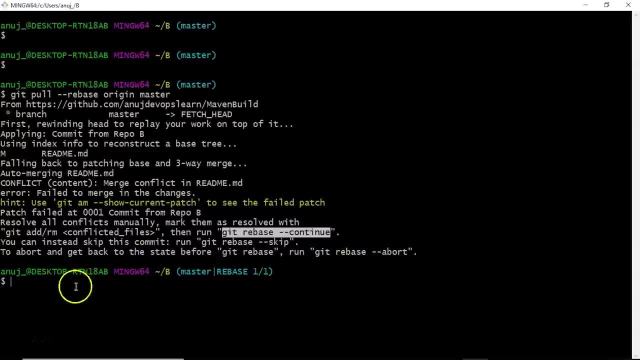 case, you can run git reverse hyphen, hyphen abort now, since we want to manage or we want to resolve this conflict manually over here. so what we need to do is that we need to open the merge tool on this one. so once you open the merge tool, from there you will be able to resolve those changes manually, and then. 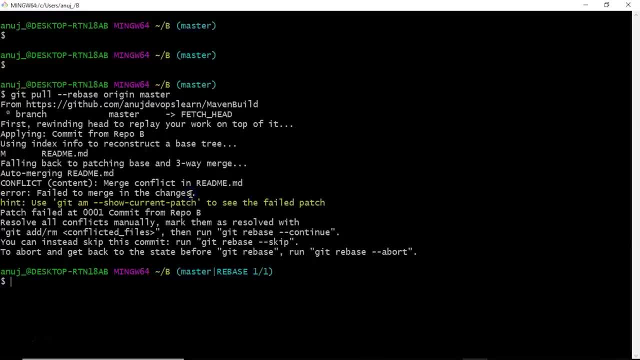 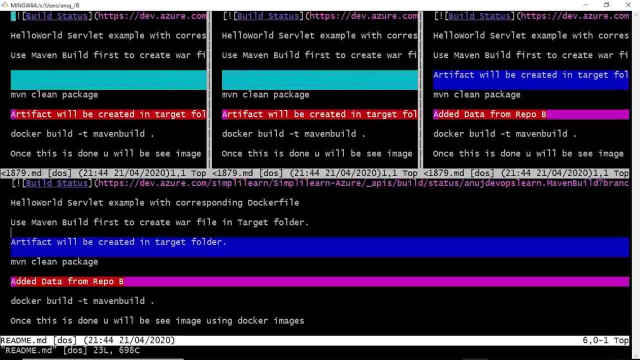 continue with the rebates. so let's go with the git merge tool here. so we are going to use the command called git merge tool now when you run this, so what will happen? that it will process, it will open the normal vi command line over here and all the files will be processed altogether. now, this is the 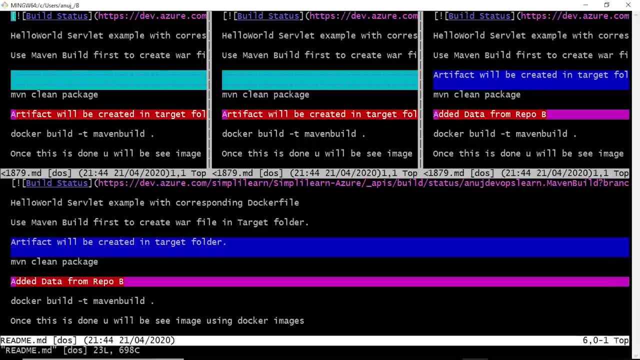 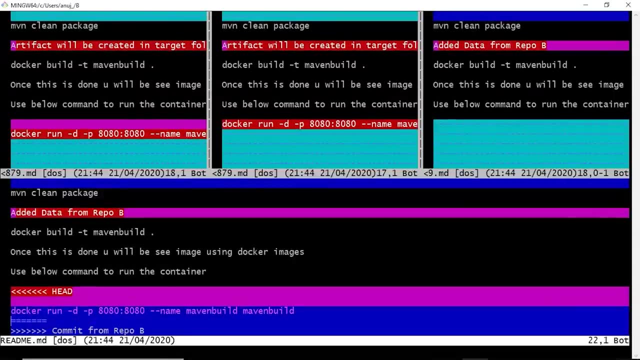 modifications, right, which is you know which is done over here. so we are just trying to see that, which particular file or what resultant file we want to configure here right now. in this case, since you are able to see that this is the final file which is present and here exactly the merge conflicts comes up, 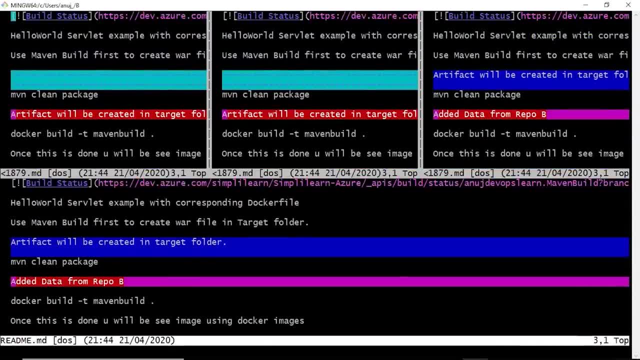 you can see that three different files are given to you in this site. so you have some files in which you added new two lines, and here you added this line. there this artifact will be there now. here you also added this particular new line instead of having this line default here. so 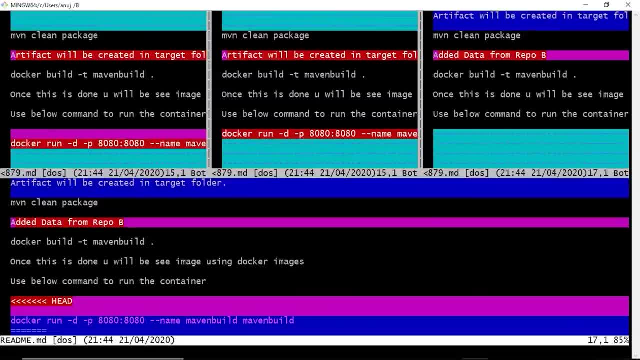 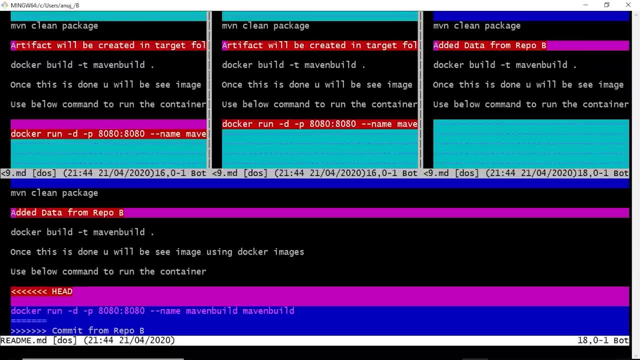 what exactly happens. when you scroll down, you will be able to see that, where exactly is the particular issue or whatever the different modifications you stand there. so in this one, if you scroll up and down, you will be able to see that, what exactly it happens. so the main area of 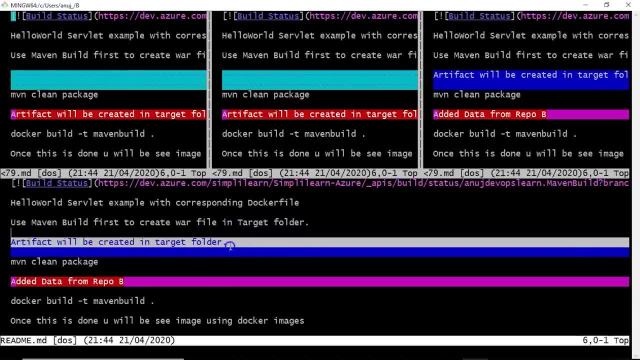 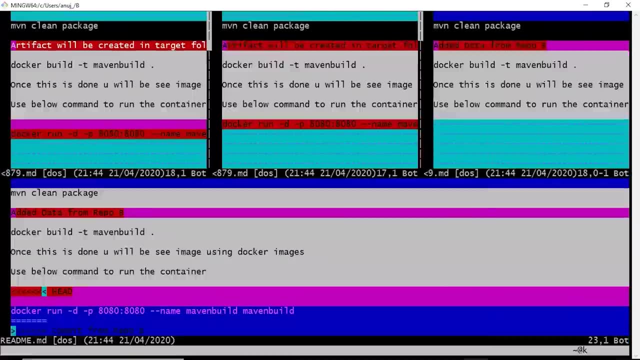 conflict is first of all this area. so this should not be there as per git, as per the normal file. but yes, if it is there. so we have to see whether we want to continue or we want to proceed with this particular specific file or not. so, yes, so I will say that, okay, let's remove this line, let's not. 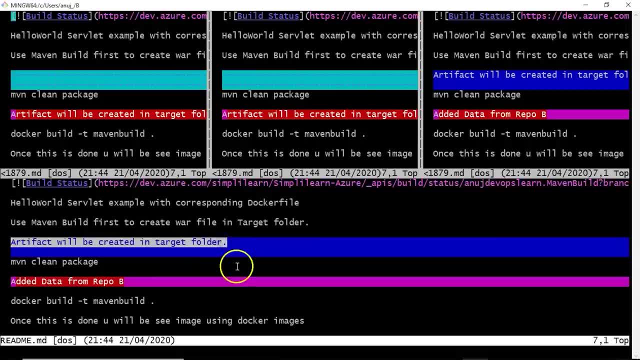 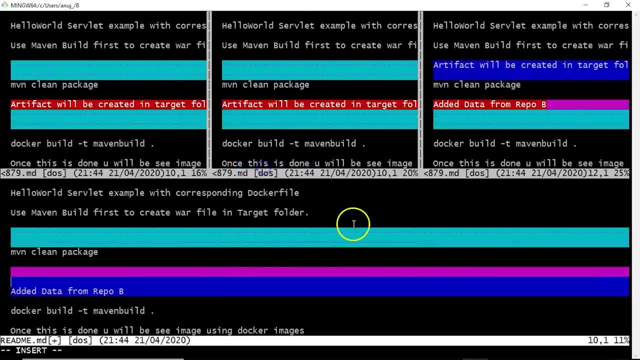 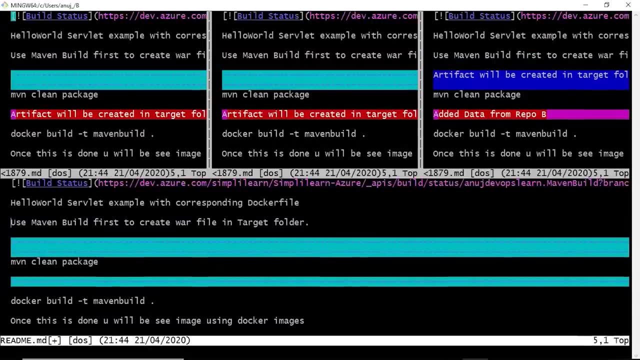 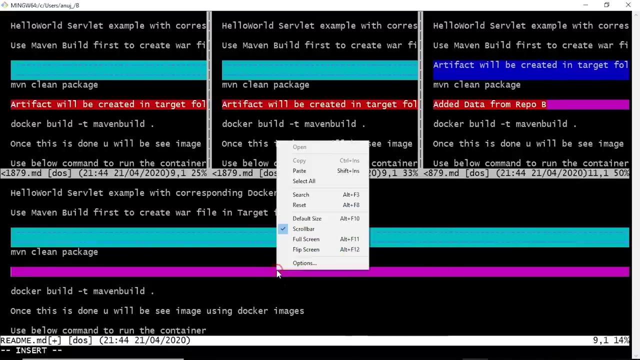 copy this line. let's delete this line here and add the line over here in this one and please, this line also from here. so this is what I am just trying to make use of here now. here I just want to have the particular line based it. okay, delete it. so this line I will. 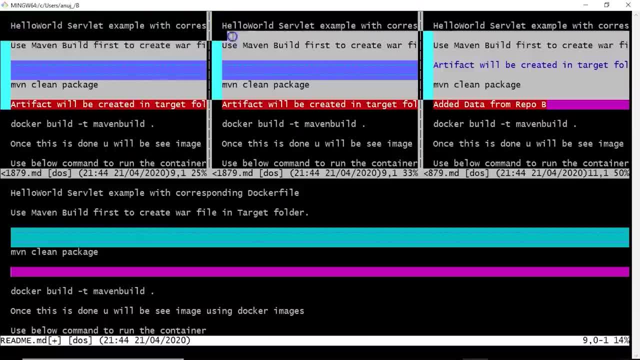 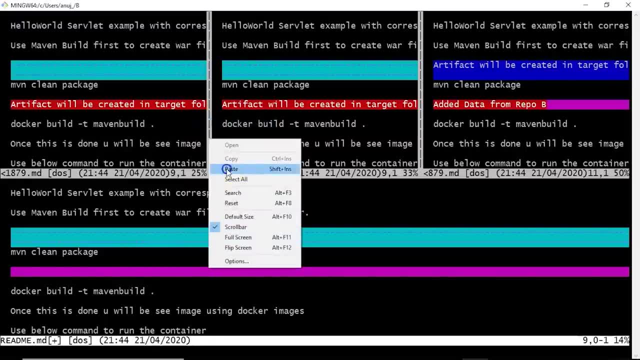 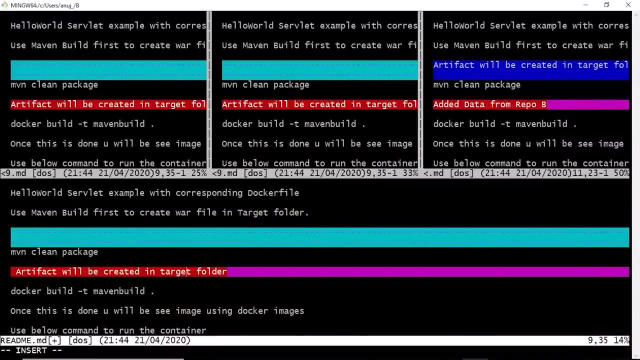 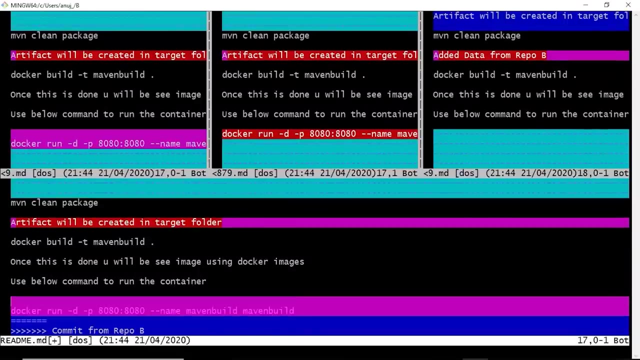 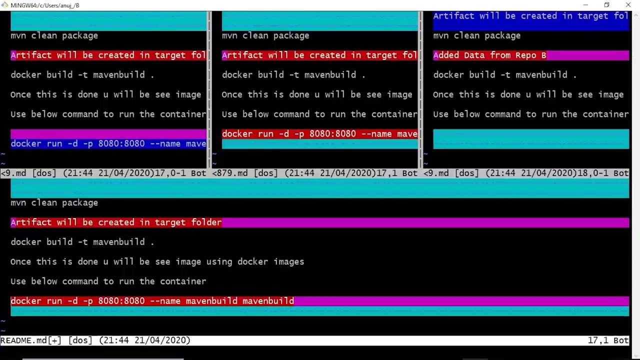 okay, so I have added this line in the final. I'm just trying to resolve this conflicts manually. I'm just editing this file here, trying to remove this one, this one, this one and this one. so this is how my particular final file looks like and I am good to go to this one. now you have resolved the. 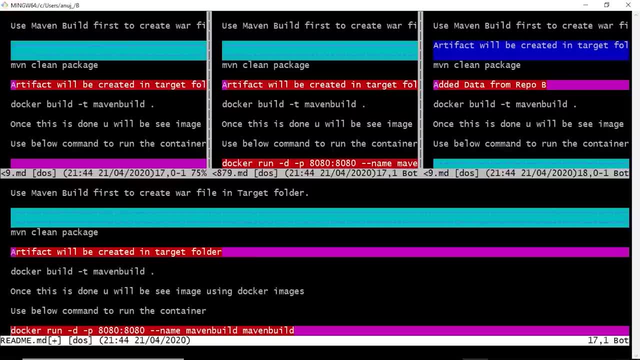 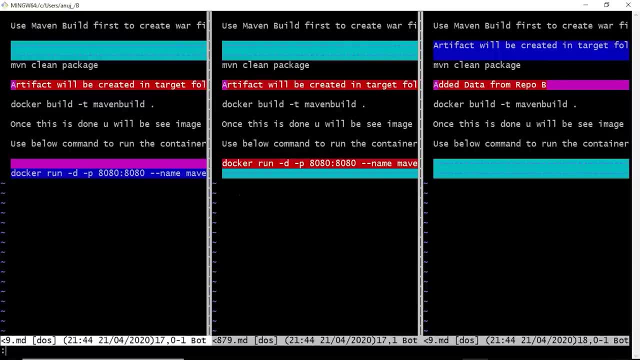 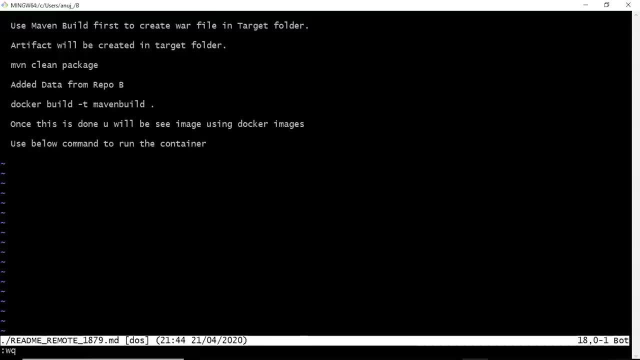 conflicts manually by doing the modification to the file. now just press colon wq, save the file over here and then close the other files also right. so this is how I have done the modifications and I have done the modifications and I am good to go to this one now. you have resolved the conflicts. 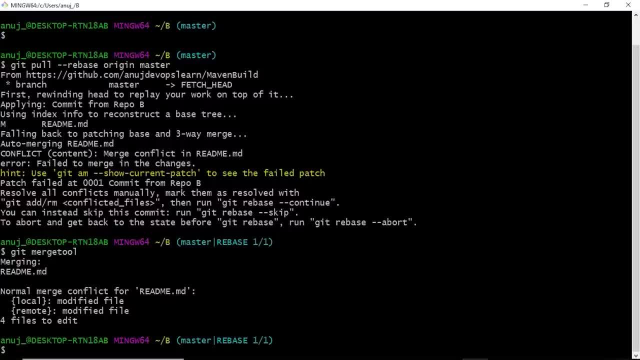 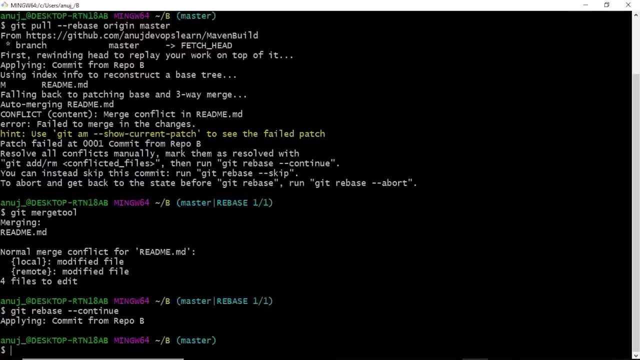 I should be able to continue further now. so what I'm going to do is, like I'm going to run command git previous. I will even continue now, once that is done. so the particular commit, which are the modifications which you have got over here. so that is something which is totally done and, yes, the 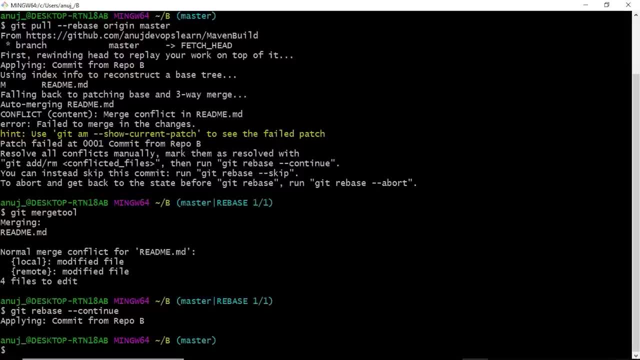 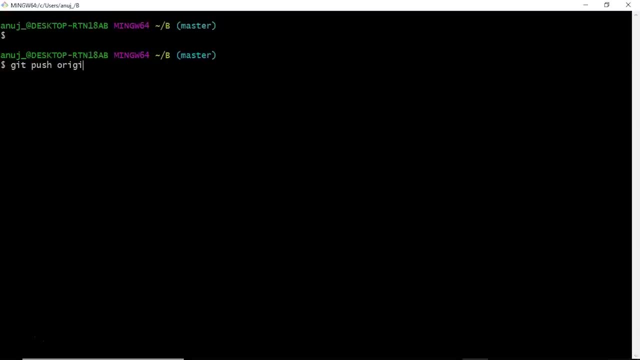 reverse is finalized over here. now again, this is the manual modifications which you have done. so you should be good to go to push to remote repository. so again, in this case, what you're going to do is they're going to run like git push. before that, if you want to check the particular git log, so you can check the particular git log. 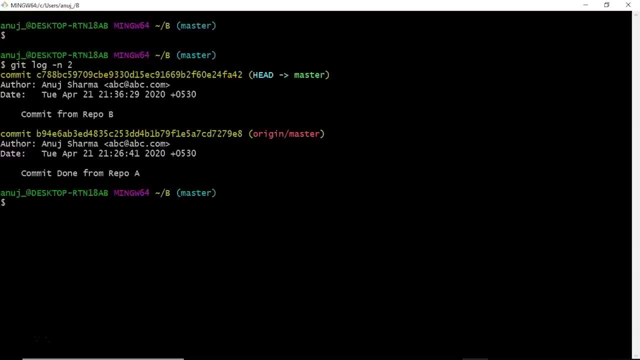 over here. so the last commit which we were try to doing like commit from repo B is also available over here. right, so A and B, both changes are present now so we should be able to push the changes to remote repository. so it will take some time to do the push. 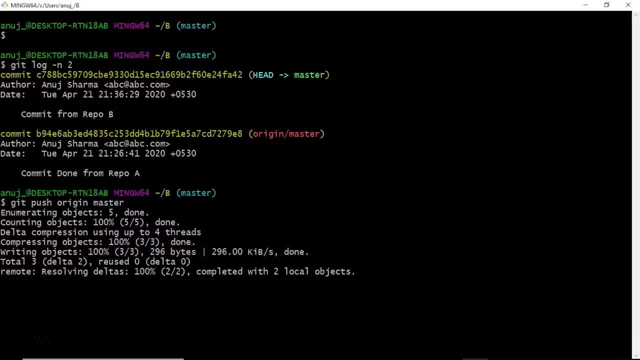 and, as you can see, it's trying to put some content. so we'll still wait for the final confirmation so that we can assure that, yes, all the conflicts is resolved and yes, that's correct, all the particular conflicts are resolved and we should be able to see both commit A and commit B in. 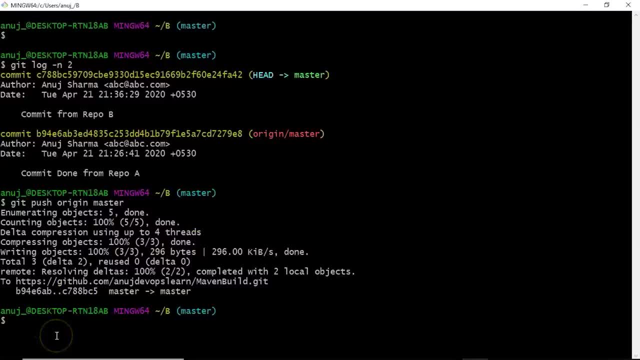 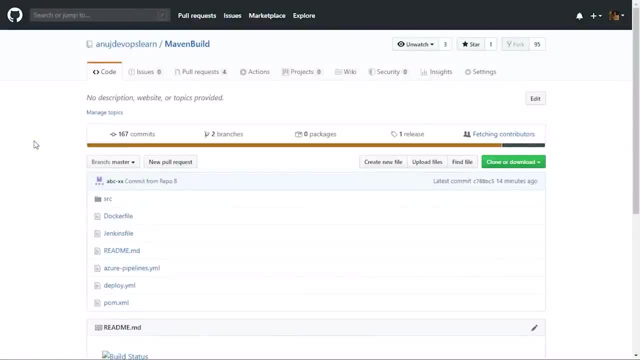 into the repository. so let's go back to the github portal and see that, if we really got those particular commits in that, so let's, when we access our particular repository on github, so we should be able to see that, uh, we have got an activity, that the commit is checked in there. 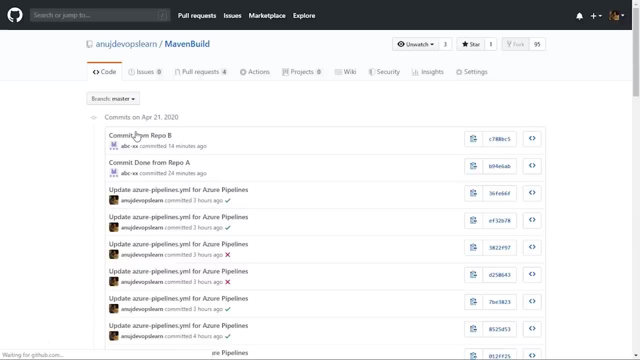 so if you go to the commits part, you should be able to see that you have got these commits can process all together. if you click on any one of the commit you will be further able to see also that what different changes you actually moved. so this is the way that, how you can resolve the 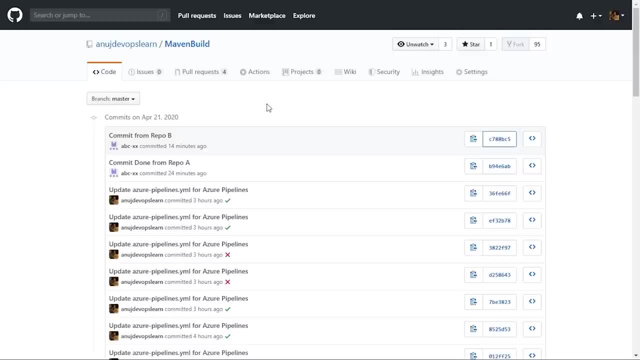 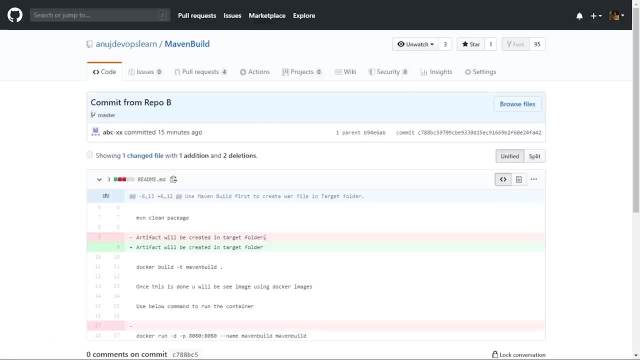 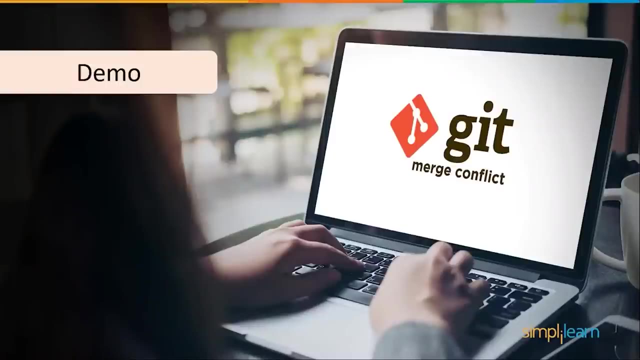 conflicts and you can uh take care of the changes from two different developers or for two different push activity. so that's it for this particular demo. i hope you liked it. thanks everyone. so we are done with the demo and we have understood that how we can resolve the merge conflicts. 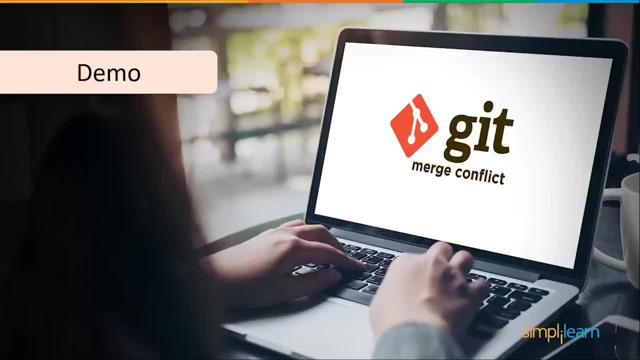 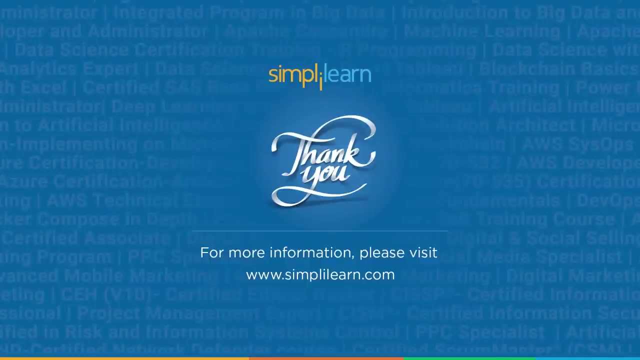 with the help of some couple of commands. now in this we really have got an understanding that how the different ways of merge conflicts really gets originated and how we can help or we can make use of some git commands to resolve those things. so this is what we had in this model i hope you really like. 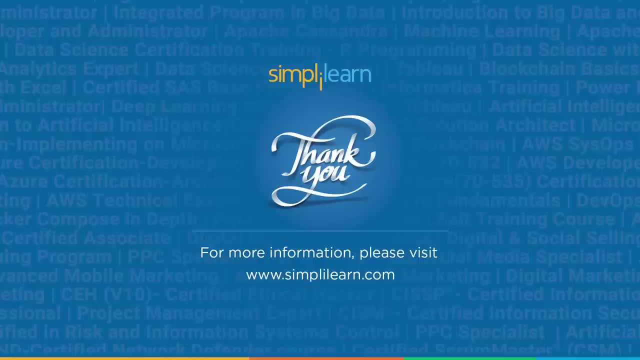 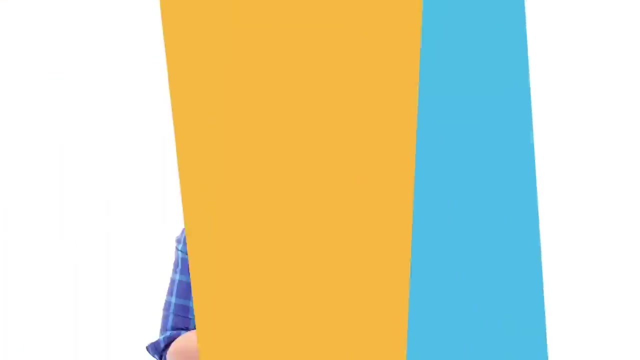 it. but in case you want to have any kind of more information, you can always visit wwwsimplylandcom here. so thanks everyone for this one you module. i hope you like it. thanks hi there. if you like this video, subscribe to the simply learn youtube channel. 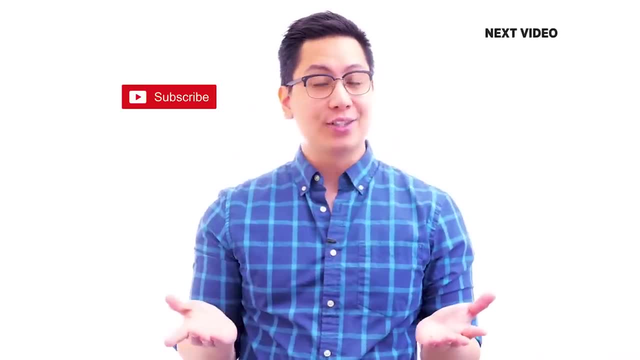 and click here to watch similar videos. to nerd up and get certified: click here.